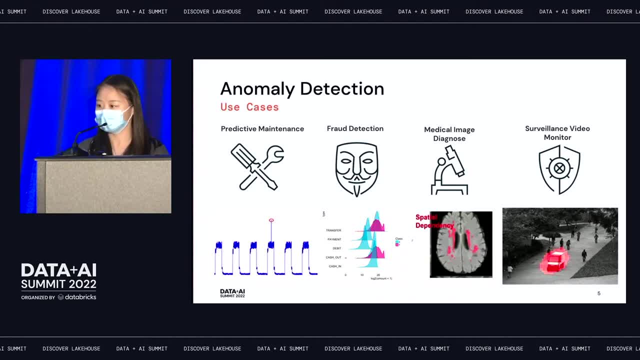 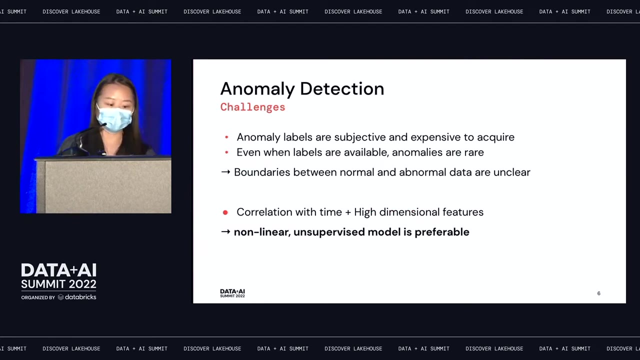 comes to those, are you with respect to structured data? when it comes to images and video processing, Anomaly detection models can also be used for image, medical image diagnose or surveillance video monitoring as well, But the common challenges for anomaly detection use cases are: first of all, anomaly labels are subjective and hard to hard and expensive to acquire. In those cases, the label has already been prepared and provided for you. Anomalies are the rare cases and underrepresented in your data set. This makes the boundary between normal data. 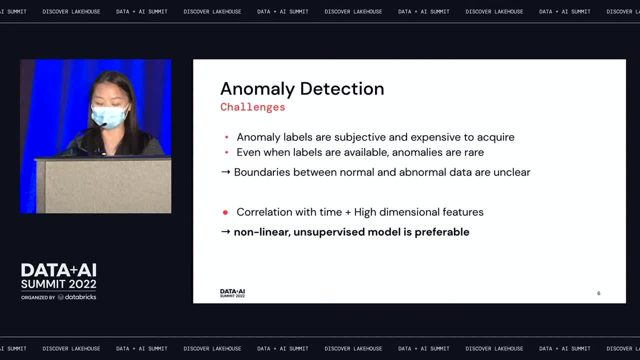 and abnormal data very subjective and unclear to define And most of cases anomaly detection usually have a strong correlation with the time domain. You want to analyze historical behavior and compare it with the current behavior to see whether there's any abnormal signals and, at the same time, 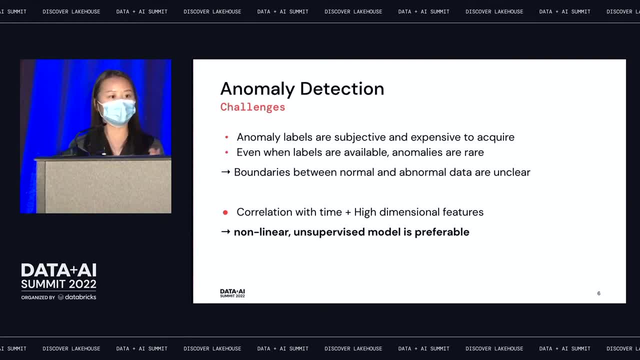 you probably want to look back a time window rather than just looking at one single instance, So that correlation with time causes high-dimensional features and making analysis relatively complicated. So a non-linear, unsupervised model is preferable. The industry has a trend and auto-encoder. 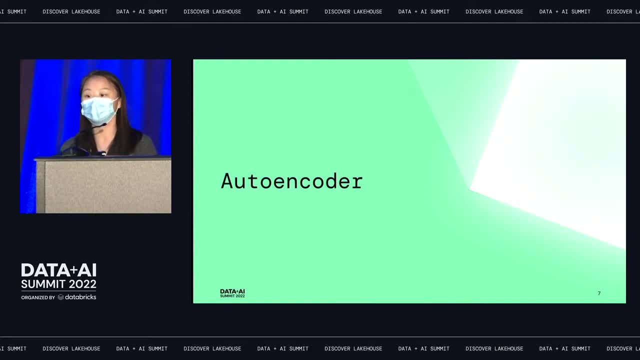 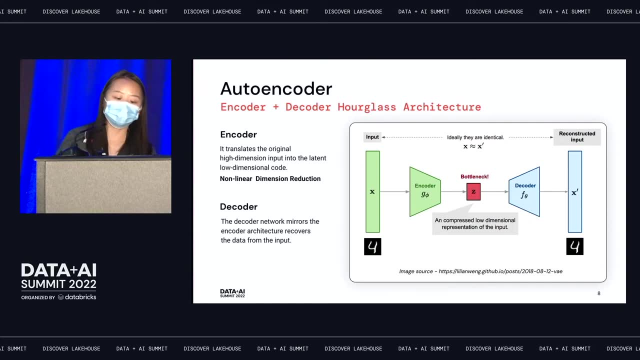 is a popular tool to use for anomaly detection use cases. Let's take a look at the auto-encoder architecture first. Auto-encoder has this symmetric hourglass architecture. It has an encoder network and also a decoder network. The encoder translates the original high-dimensional input. 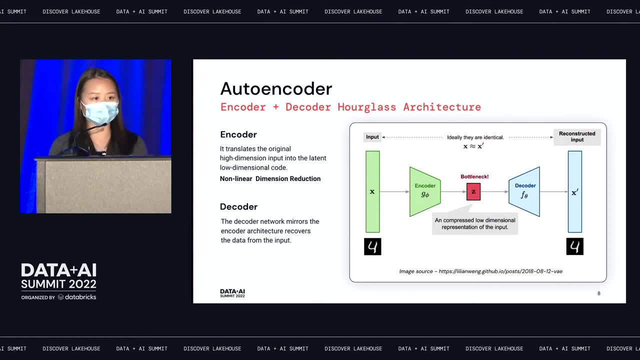 data to the bottleneck layer and produces the lower-dimensional latency vectors. It's a non-linear dimension reduction, if you think of it that way, And then the output from the latent space will be input to the decoder and then decoder will try to mirror the architecture. 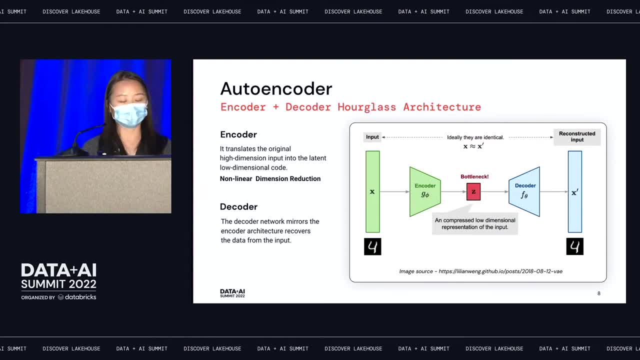 of the encoder and reconstruct the data from the input data You can use very. you can have very flexible architecture choices when choosing. when building auto-encoder. You can use dense, CIN, LSTM or build customized layers for your architecture. And the latent space is just a non-linear representation. 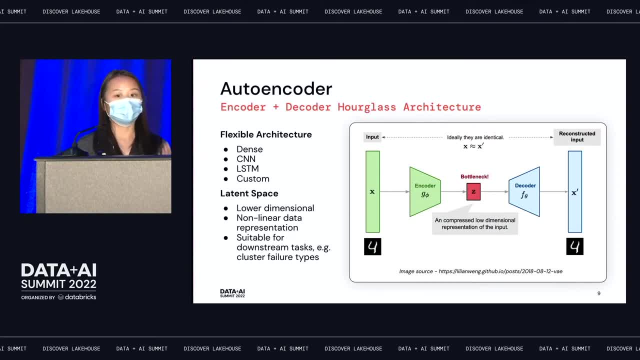 of your input data. Similar as any dimension reduction algorithm will do, the latent space produces embeddings of your data. Those embeddings thus can be used for downstream tasks like clustering your anomalies. You can also use data types or clustering your healthy data types. So the steps usually we would do, we would perform. 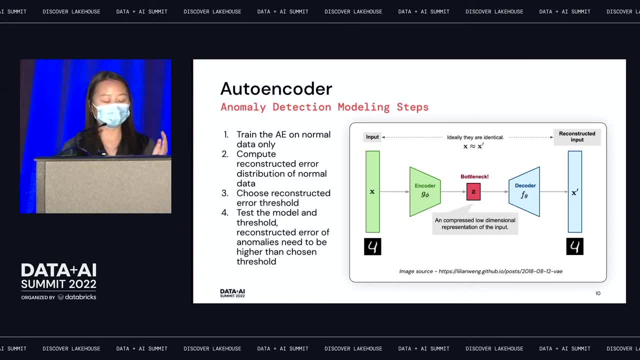 for auto-encoder modeling are listed here. We will first build, like. of course, you will first understand your data, trying to get data insights, build the right features, cleanse your data and then build your model architecture. The selection of model architecture is a. 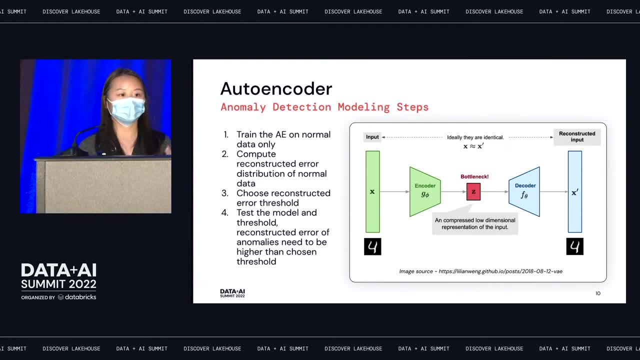 common discussion and we will have soon coming slides talking a little bit more about that. Assuming you already have your network being constructed and ready to train, those will be the following steps. We train auto-encoder on normal data only and we'll compute the reconstructed error distribution. 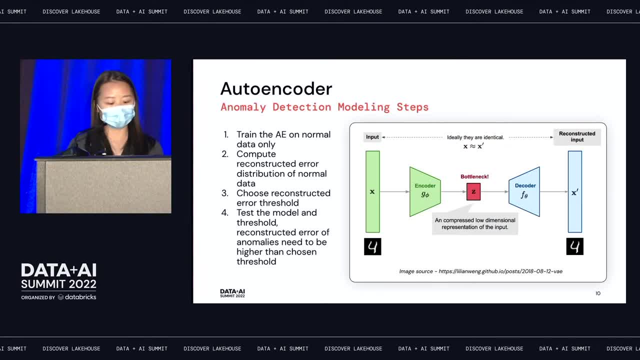 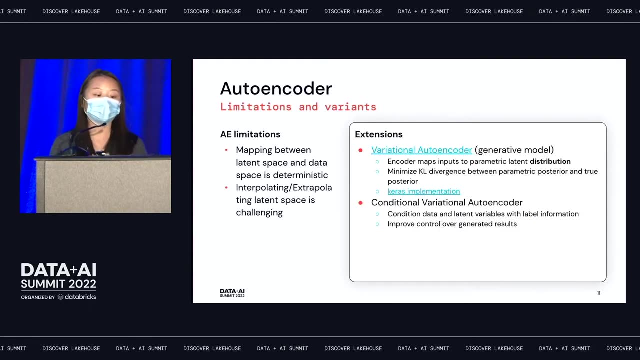 of your normal data. Once we have that information, we'll try to choose a proper reconstructed error threshold, and anything about that threshold coming from the new data will be considered abnormal data. There are limitations of the classic auto-encoder as well. The main limitation is that auto-encoder is a deterministic model. 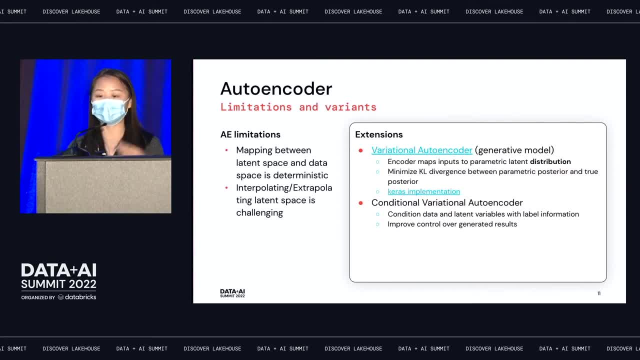 and the mapping between latent space to the data space is deterministic, making the interpolation and extrapolation from latent space back to the input space or back to the original dimension challenging. So this is to say, auto-encoder is not a generative model If you want to generate new data from the latent space. 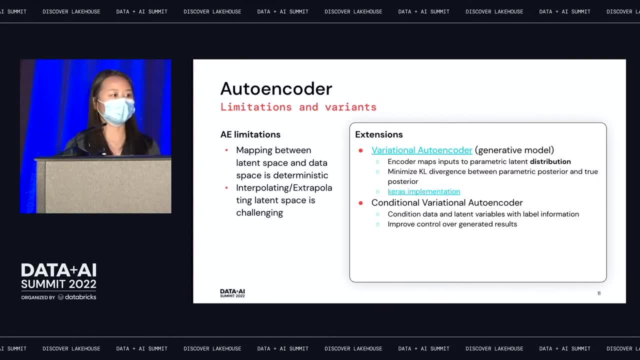 this is not the right choice. Depends on your use cases. There are some variations you can use to make it more generative or to have even more control of how to generate the data. A few options I have listed as extensions. here is variational auto-encoder. 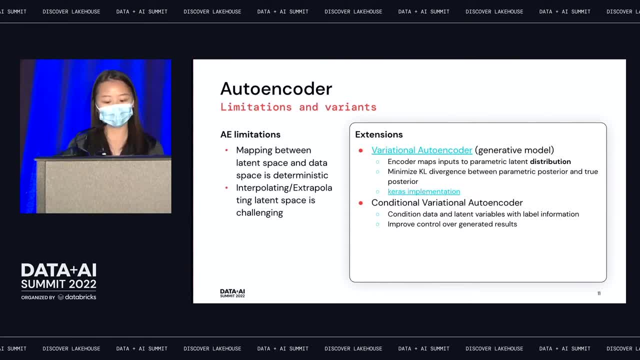 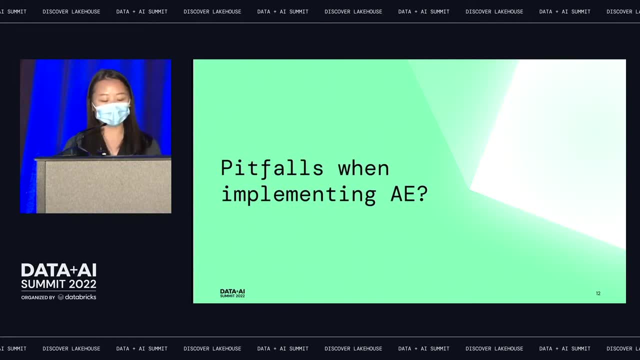 and conditional variational encoder. Feel free to check out more information on those and we'll try to talk about focusing on the implementation of auto-encoders. So we have covered some basic concepts, but when it comes to implementation, what are the common pitfalls? right? 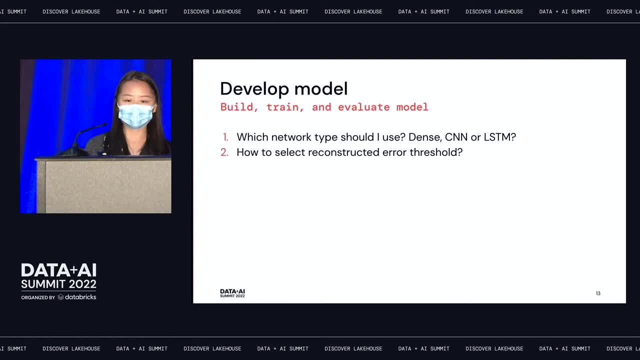 The two most common questions I have experienced when working with auto-encoder models is, first of all, what type network should I use? Should I use a dense network or should I use CIN or LSTM? And the second is: how do I choose the reconstructed error threshold? 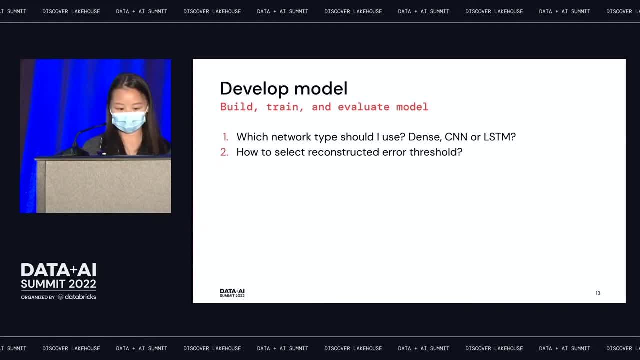 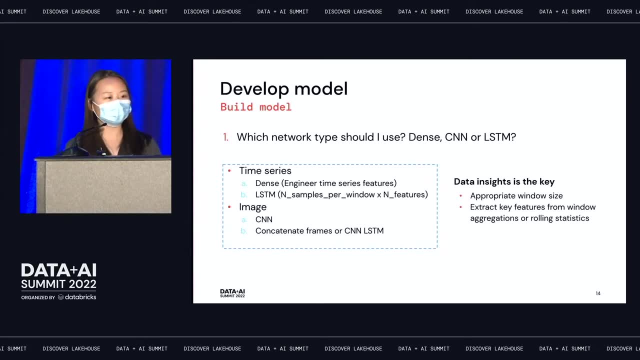 So let's try to tackle them one by one. For the first question, what type of network should I use, My opinionated answer to that is: data insights is key. Let's be data centric, trying to pay as much attention as your data, spend as much effort. 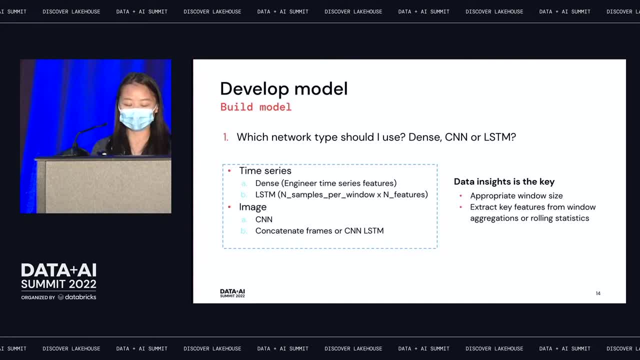 in your data analysis before you start to build out models. Some straightforward approach in machine learning or deep learning models still applies. For example, when you have image computer vision use cases. it's very straightforward to choose a CIN network, But at the same time, what if you want? 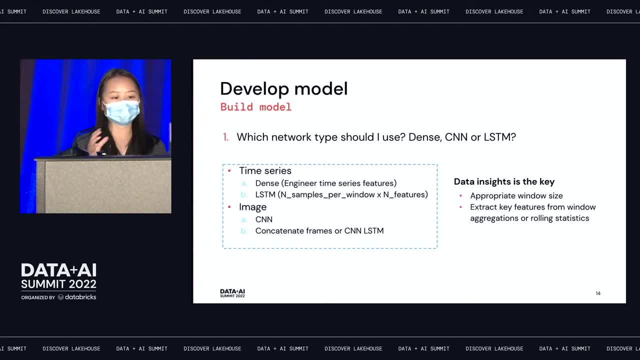 to concatenate multiple images together. Do you want to? Do you want to select a subset of one image, concatenate them? or do you want to analyze the correlation of time series between those multiple frames? Then, in those case, you need to choose between like: 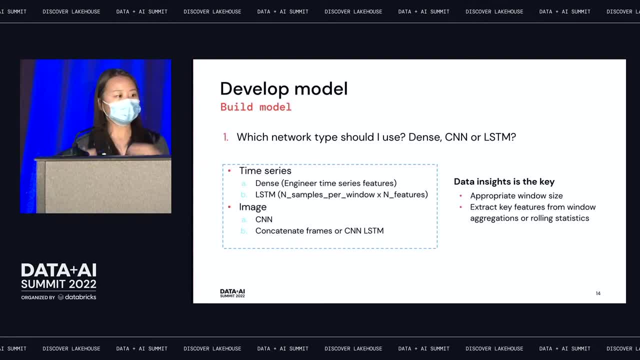 concatenated frames or CIN LSTMs, Similar in time series use cases. we can build dense layers as your architecture design When you have like good feature engineering. you've selected the right window size, being able to extract the most critical information. 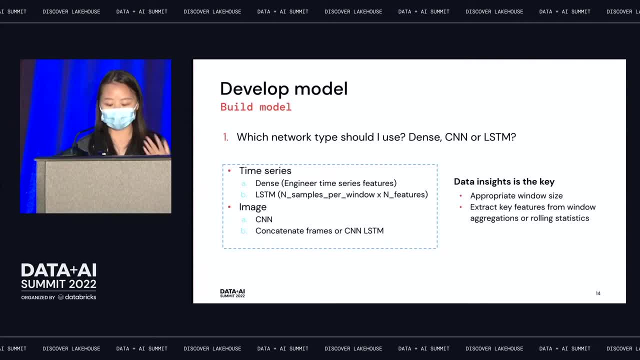 from your aggregated statistics or rolling statistics. On the other hand, LSTM could be a possible solution for time series applications as well. You just need to think about the trade-off between the training time computing resources and model accuracy and model generability. 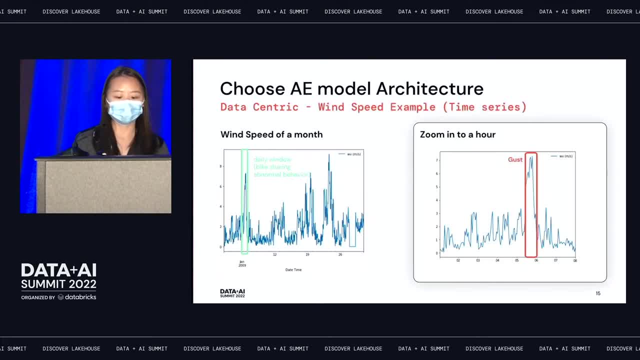 To elaborate a little bit more on that, I have this example using wind speed a shared feature for two different use cases. We have the same raw wind speed data for two separate use cases When we're trying to detect abnormal user behavior of a bike sharing app. 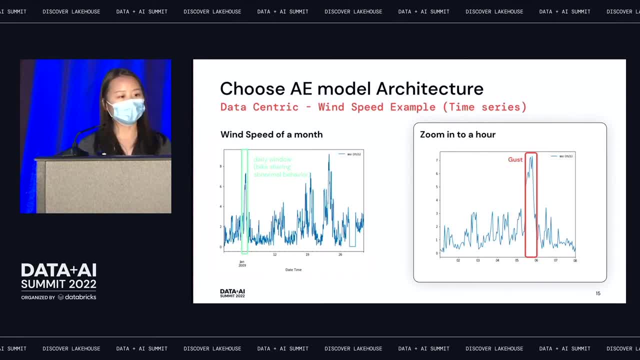 probably aggregation of that maximum or medium wind within an hourly window or even a daily window is appropriate contextual information for your model. But on the other hand, if you are trying to do a predictive maintenance case, trying to see whether your machine or devices has been behaving normal with respect to the wind gust, which happens within like a minute's level, 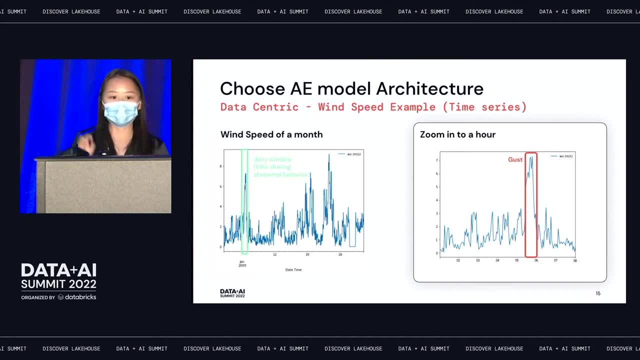 then you need to choose, like a window size, which need to be as fine as one minute, to run the analysis. So think about how you can use your data and extract the feature that best fits to your use case. That's way more important than choose the proper architecture or network. 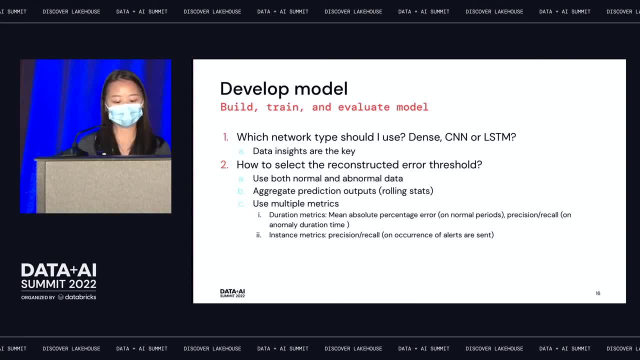 All right. When we come to the second question, how to select the reconstructed error threshold- um, there are a few things we can, a few tricks we can apply here. First is like: make sure that you have the right data. So if you have the right data, you can make sure that. 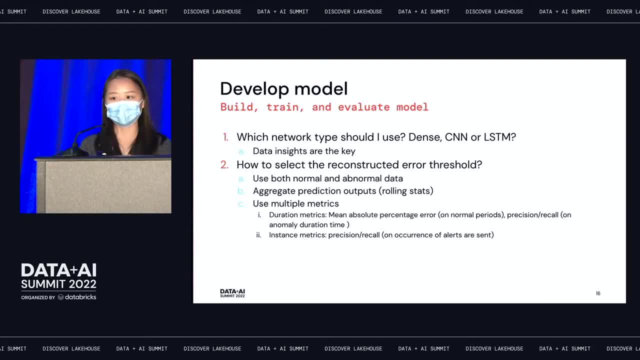 you have the right data. So if you have the right data, you can make sure that you have the right data. So if you have the right data, you can make sure we use both normal and of normal data in the evaluation process. So when, when we train our autoencoder, we train it on the normal data only. 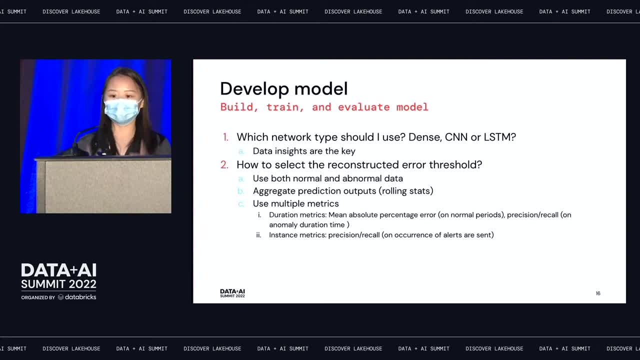 but that's not throw away the abnormal data and fully use it in our evaluation process. So this way it will give you a clearer decision boundary between the normal and of normal behavior And, at the same time, instead of using, like raw, reconstructed error, as you know. 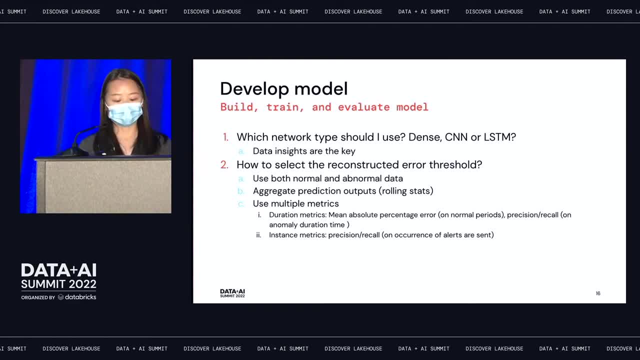 as your threshold. think about using uh aggregated results. It could be a min value within a time window you selected. So, for example, you probably consider your uh devices is failing when uh the threshold, the reconstructed error threshold, min value within an hour has reached one certain 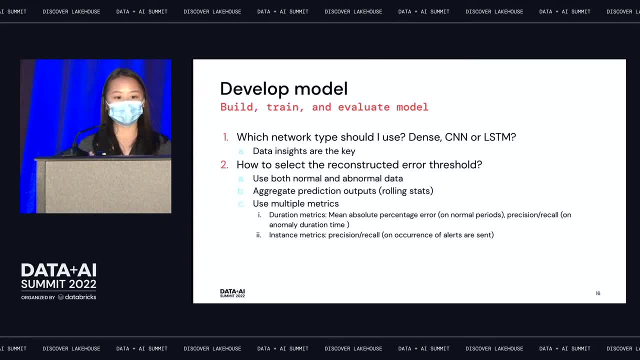 threshold or in some cases it could be accumulated rolling statistics- right, It could be a great gradual change to your devices and you accumulate the reconstructed error throughout the historical to current time. When the accumulated error reaches a certain level, then you consider this is like a 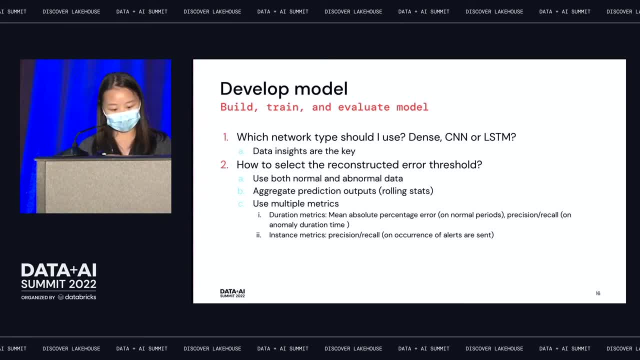 time that trigger that failure: detection, detection. And the third trick here is to use multiple metrics. So, uh, when we build models and train models, we rely on per sample instance, but when we do evaluation we can do both duration level metrics and instance level metrics, Duration level metrics, example. 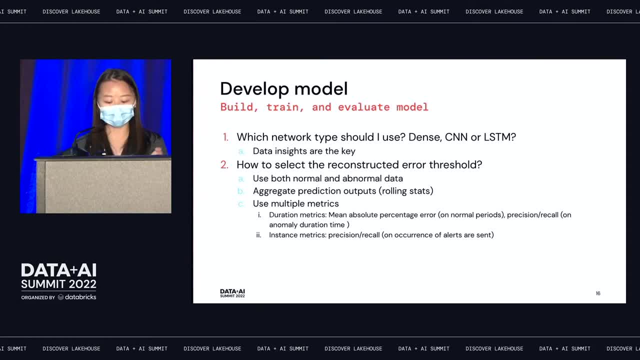 include min average, uh, min absolute percentage error on the normal period. So you have a long period, say one year of period, where your machine has behave like normal, but then your sample period could be at 10 minutes level. So within this whole one year of data you have a lot of. 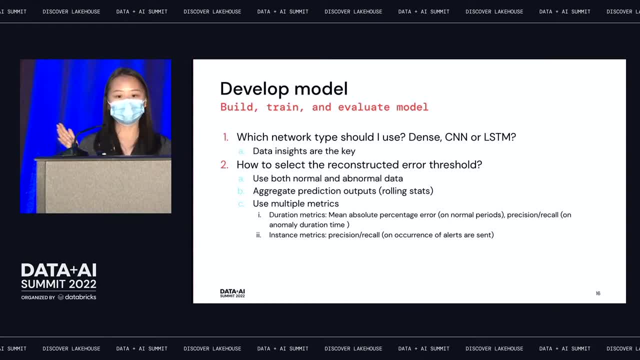 samples to uh test your model on those normal data to see, within this normal duration, how many times that reconstructed error has uh, that reconstructed error metrics you choose, has been above the threshold giving you a false positive alarm. Or, on the other hand, you can also compute the 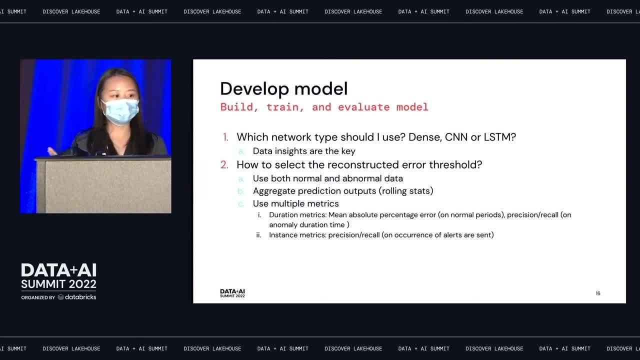 duration metrics at abnormal period. Same thing. you taking that period as considered as your metric base and only on the same time. you can also do like instance metrics. So in the past year your device has failed three times and applying this model to your historical testing data. 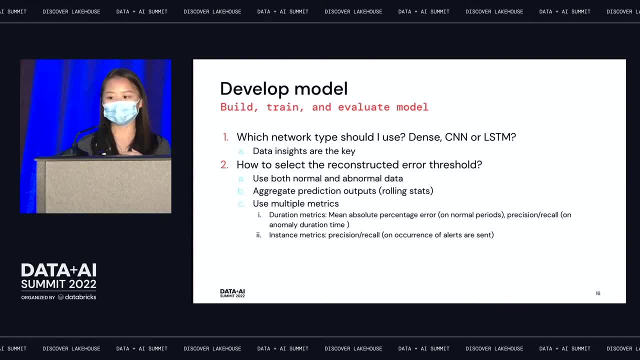 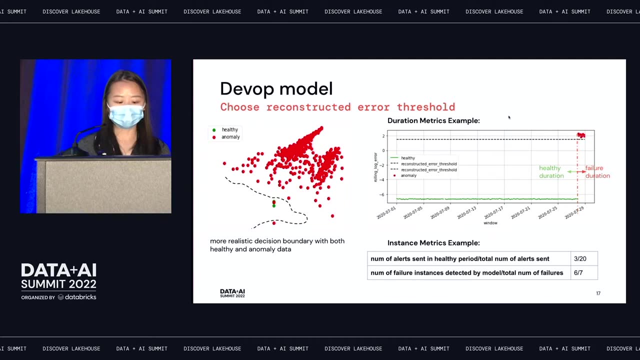 how many times it can detect the failures can be another metric to use to truly evaluate the overall performance of the model and select the correct threshold. All right, to summarize a little bit: using both normal and abnormal data in the reconstructed error threshold choice will help clarify the decision boundary. 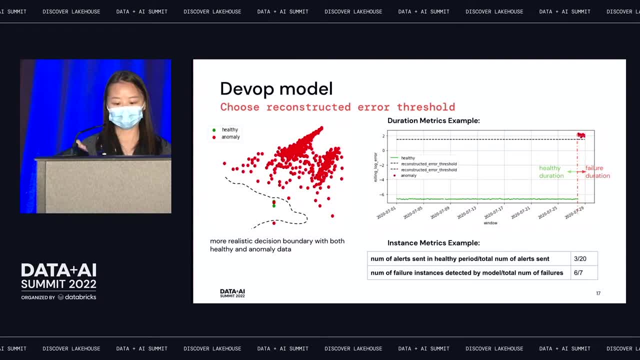 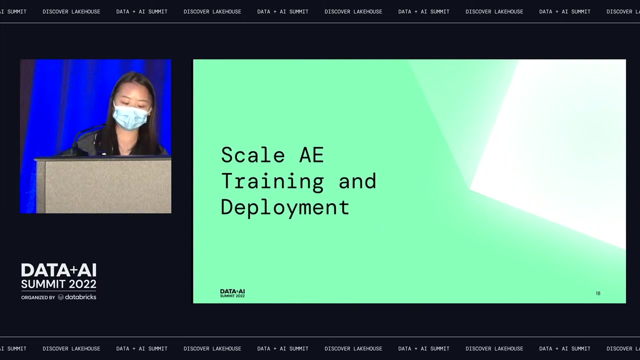 between healthy and unhealthy data And a few. when selecting metrics, we can use both duration metrics and instance metric and build that in your reconstructed error threshold selection choices. All right, Now let's talk a little bit more about how to scale anomaly detection training. 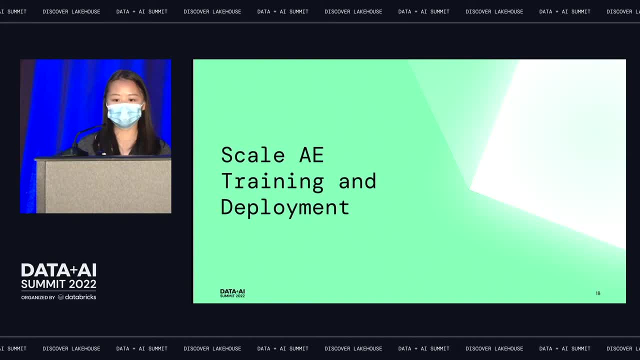 Say you have a group of devices, Is there a way to run or train one model per group instance in parallel? And once we have that- multiple models per group instance- how do we make our deployment easier? Do we deploy one model? Do we deploy the multiple models? so in the end, 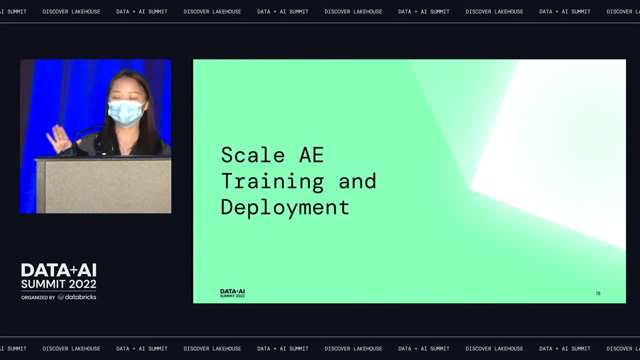 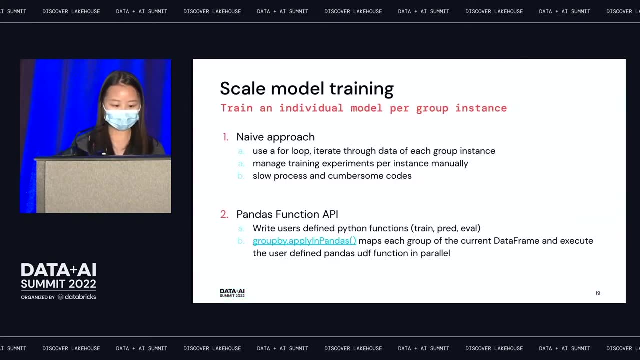 there will be multiple models running in the back end and the user need to properly choose which model to use when applying to the new data, Or how do we make this easier? So, again, the naive approach is we can use a for loop every time. we just iterate through your data. 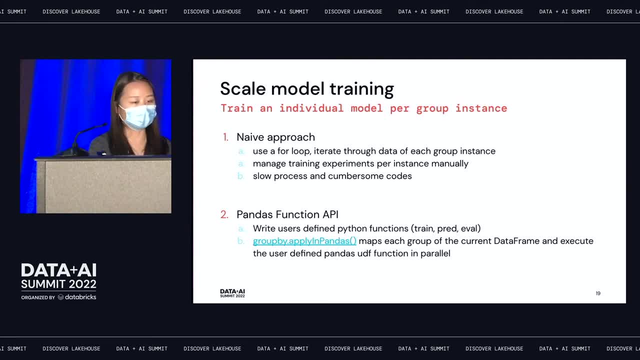 in the training process and find the segment of data for each group instance. And then we got to manage the training experiment, per instance manually and find the model, per instance through an iterative approach. The smarter way to do here is to use Pandas function API. 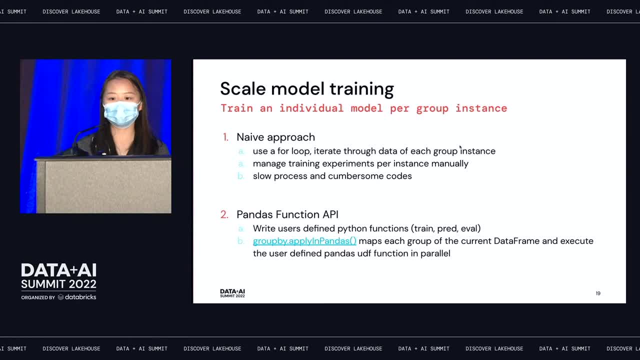 We will write user-defined Python functions for the training process, prediction process and evaluation process And we'll use a group by apply in Pandas, which is mapped group by Pandas UDF to the entire data frame and being able to execute the user-defined Pandas UDF. 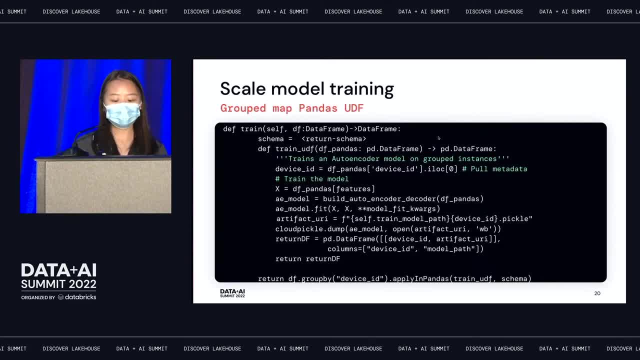 in parallel. So this is a quick code snip And we'll get to code demo soon. Basically, you will have your training function here, And this training function is taking a Spark data frame as input And what it returns is a group byte results. 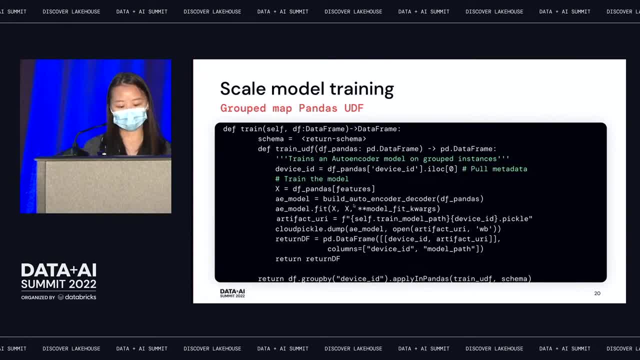 So your data frame will have the data coming from all the group instance. But what we are doing here? we're going to group this data frame by the key, which is device ID in this case, and then apply this user-defined Python UDF. 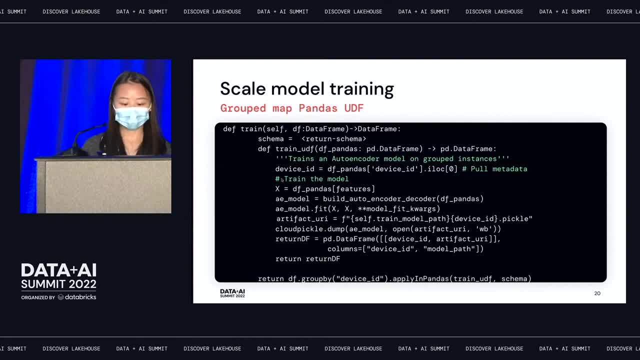 And what this Python UDF does in the end is it will basically take the data, per instance, and then build this auto-encoder model, train each auto-encoder model per instance and save the model information from the training process to return data frame. 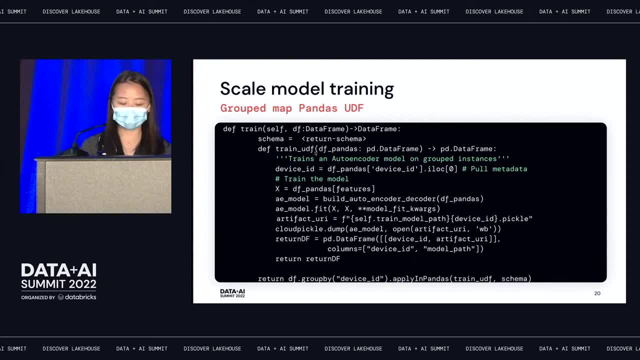 So, if you are not familiar with Pandas UDF, basically Pandas UDF need to take two key inputs. First one is the actual Python Python function And then the second one is the return schema. That's why here, when we actually 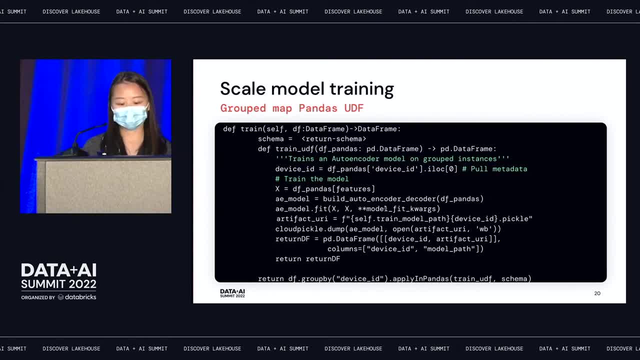 return the training results. we need to provide this customer-defined UDF and also the return schema. You can see that the return is basically our concatenated information about the trained model, per instance, And we can take a deeper look when we get to the demo. 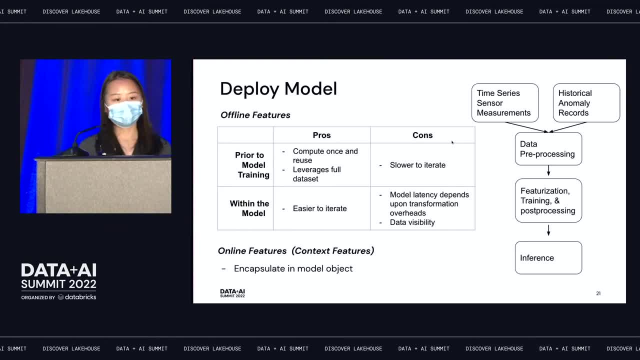 session. So now you have your model, We have your model being fully trained. How do we deploy those models? So the process for anomaly detection is usually you have some time series sensor measurement and you have historical anomaly records. We need to merge the information together and run some data. 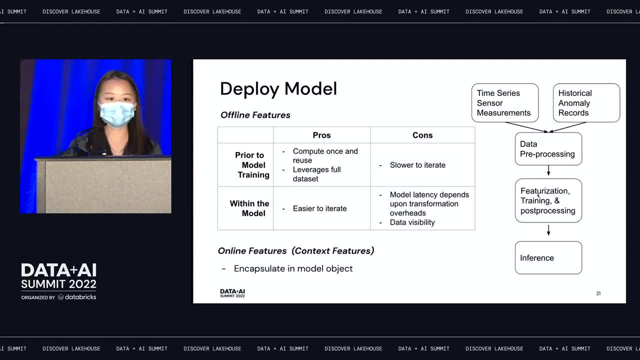 pre-processing and get visualization, training, post-processing done. And with all that model being processed and ready, we need to go back to the inference pipeline. So the model might have both online and offline features. So online features are features you can pre-compute it. 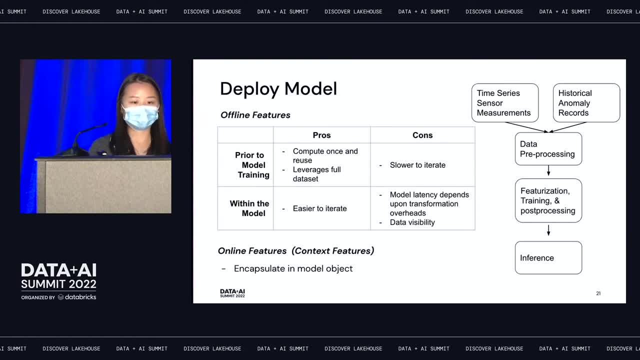 So whether to apply those offline features prior to your model training or within the model training have pros and cons for both. So if you have feature processing prior to model training, you basically compute the features once and reuse it. A common way is to write it to a feature store. 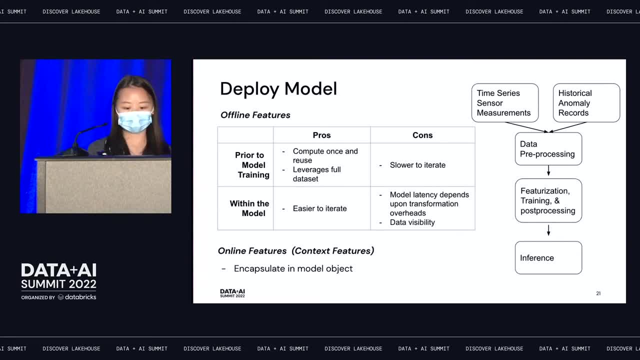 and then later ask the model to retrieve it from feature store. It's slower to iterate, but you can utilize the full data. and you can utilize the full data and compute just only once. On the contrary, if you compute the features within the model, 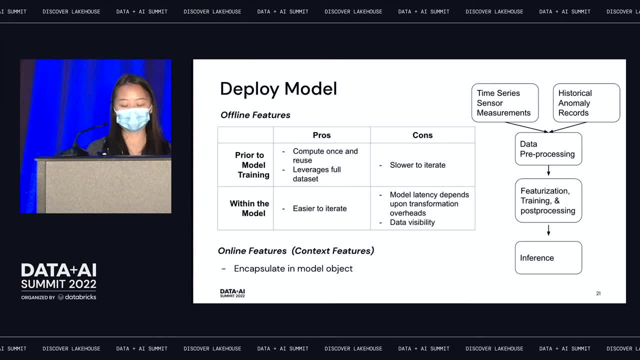 it makes the model iteration easier but also increase. model latency depends on transformation overheads and data visibility. So for this demo we're assuming all the visualization is done ahead of the model and there are no features. we're going to compute on the fly. 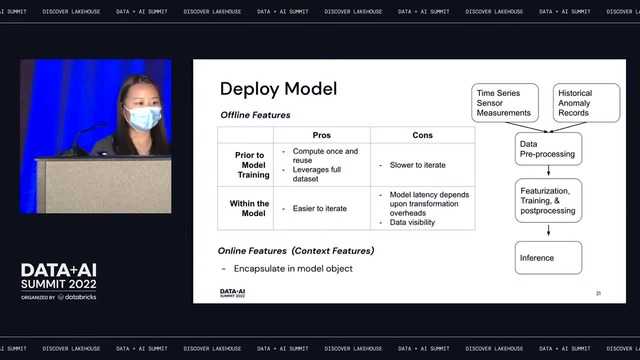 But in the case you have features that you need to compute on the fly- a quick example would be something you only acquire at the inference time, right? For example, the current Okay, Information about a device can be an online feature, Then those online feature has to be encapsulated within the model object. 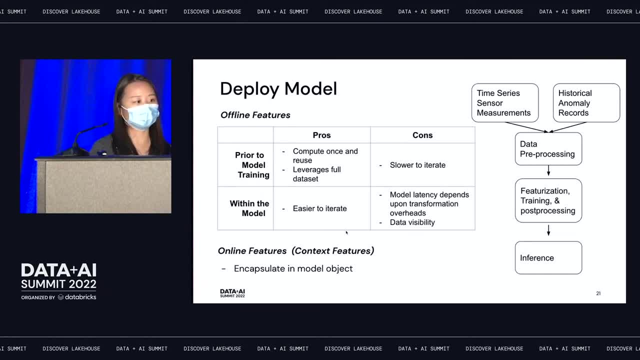 And what we're going to show is that we want to. once we have this model ready, we want to incorporate it together with the entire data pipeline. If you have your data pipeline to ingest new coming sensor data, how do we add the final step of machine learning, prediction and being able? 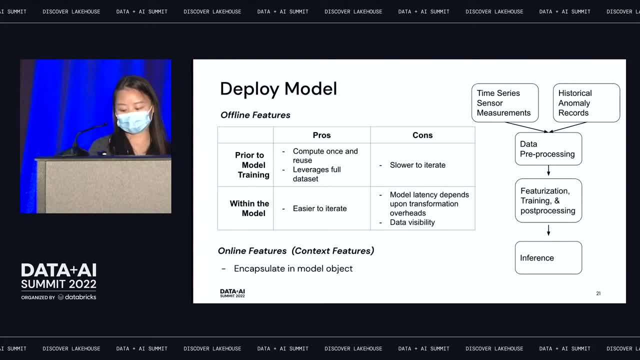 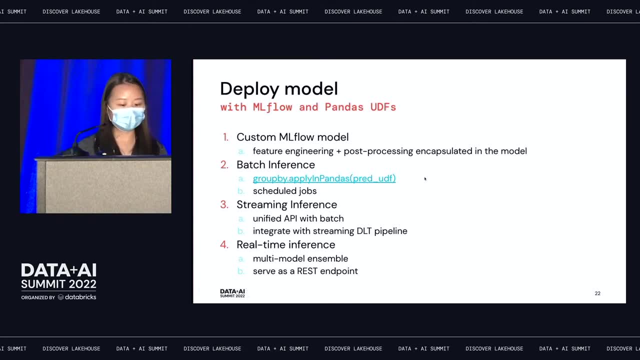 to save the prediction result back to the data lake. Here is a quick summary of what we are going to demo. We will build a custom MLflow model that will package the feature engineering and the post-process steps in the model, And then for batch inference we'll use Pandas UDF again. 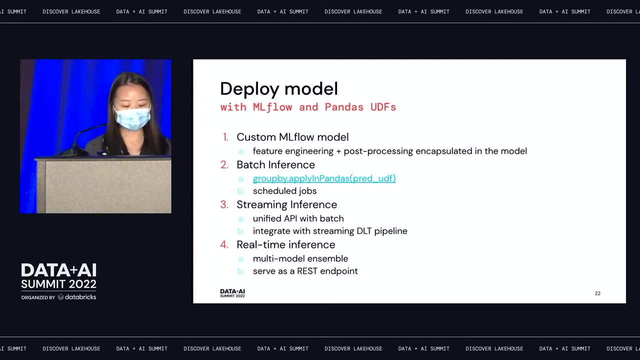 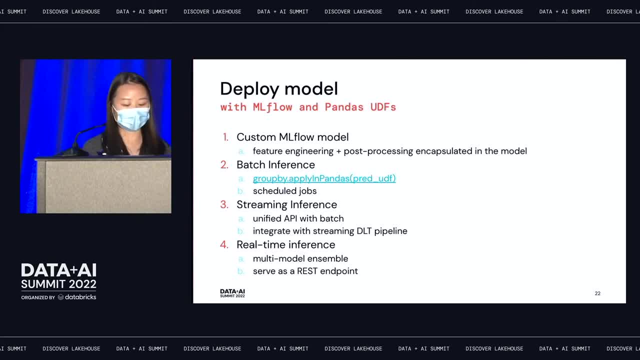 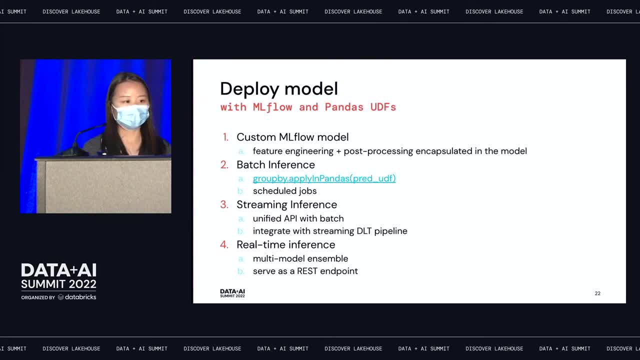 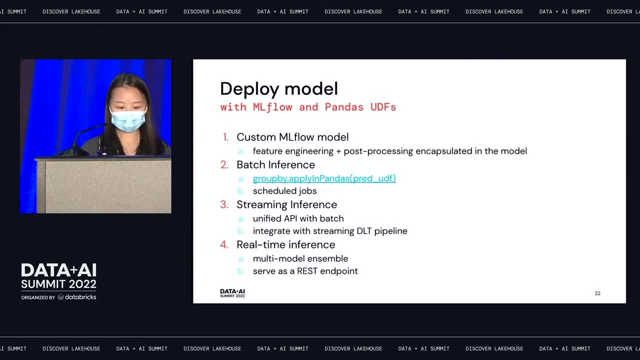 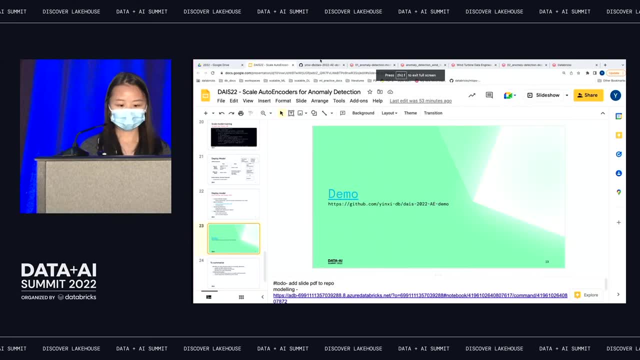 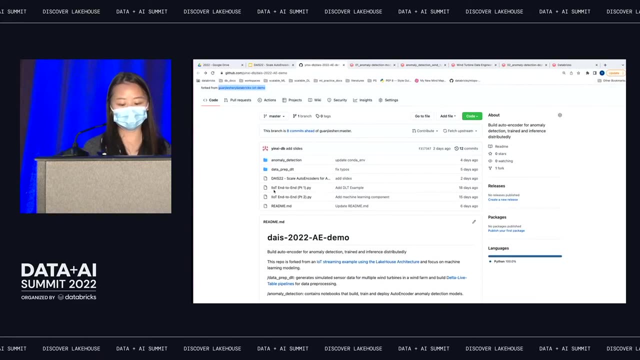 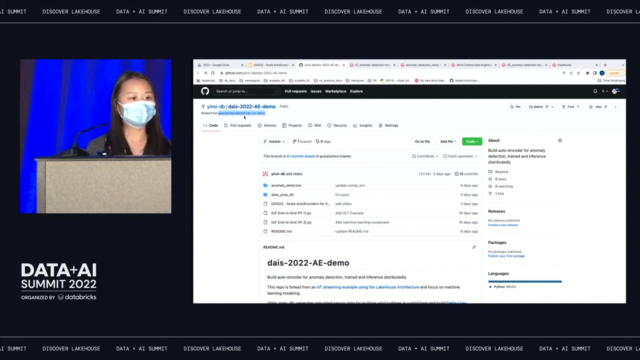 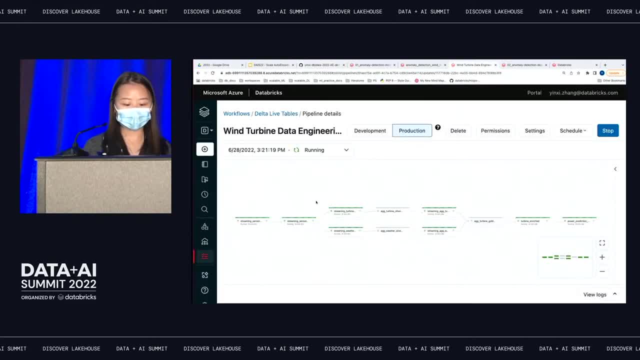 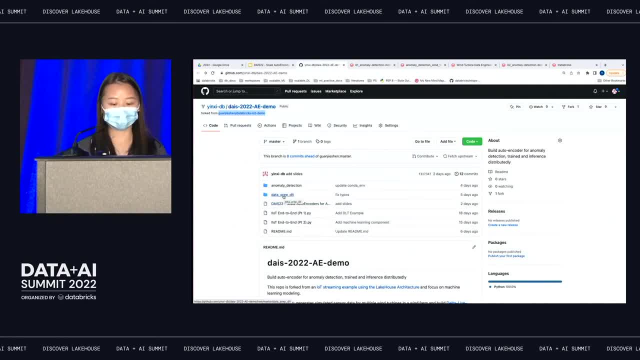 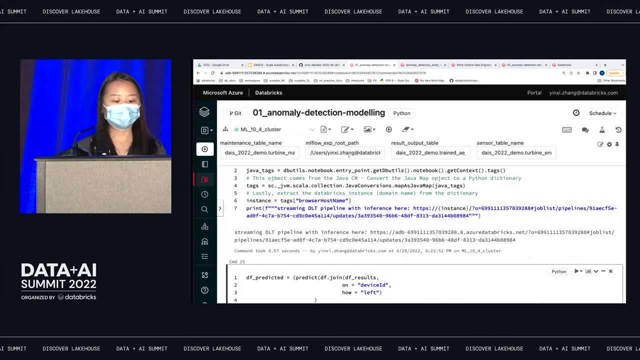 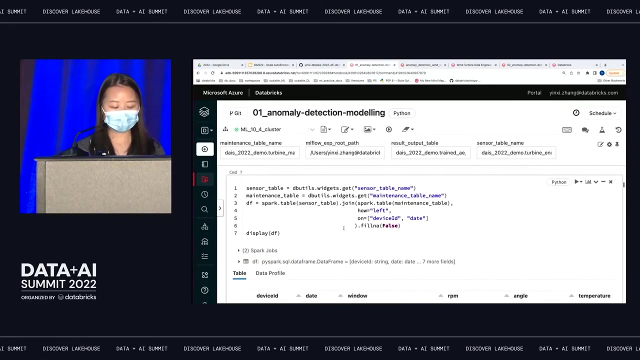 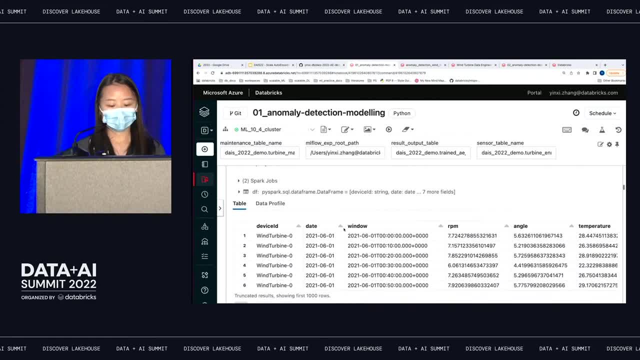 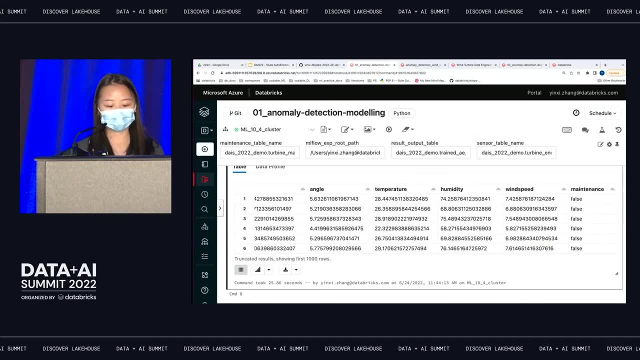 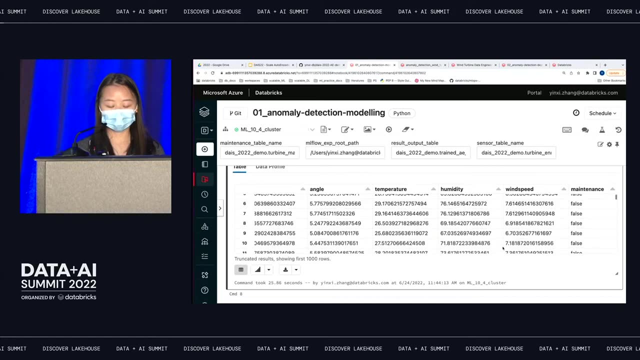 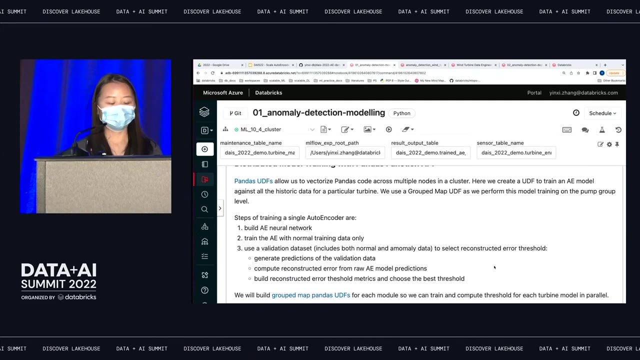 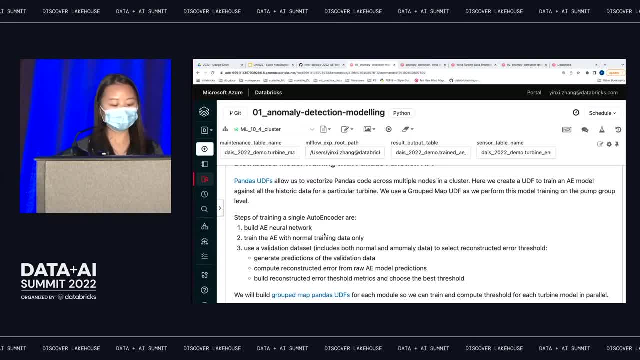 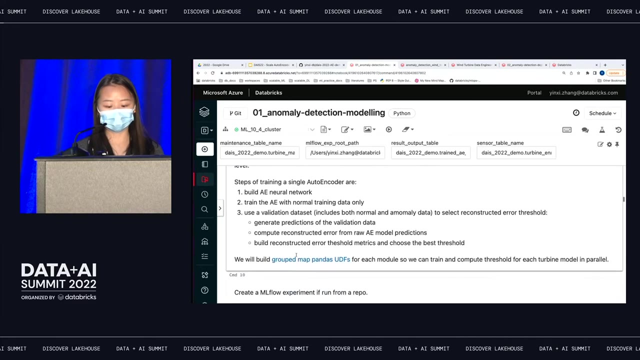 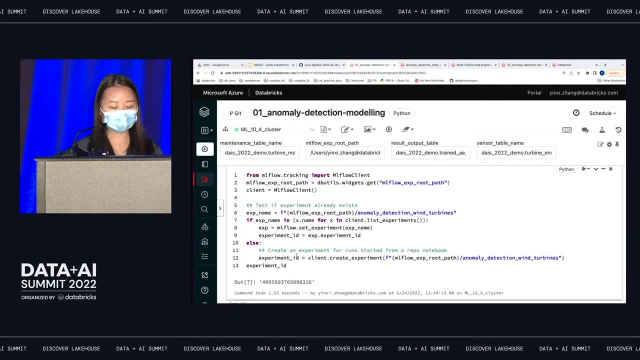 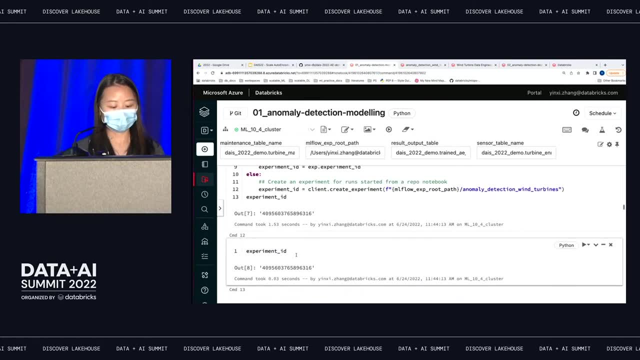 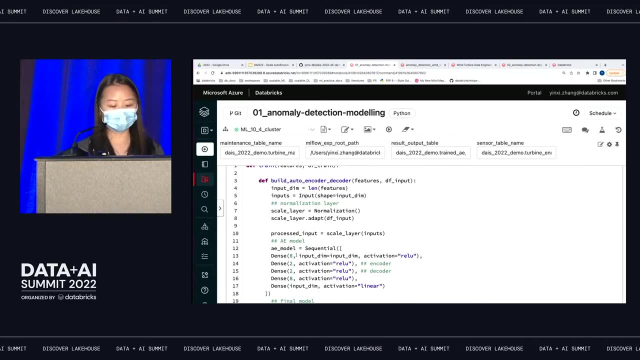 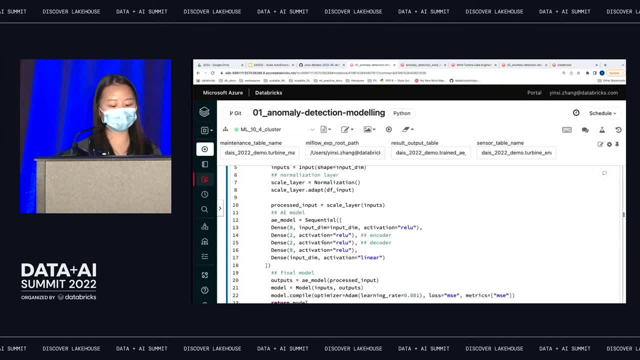 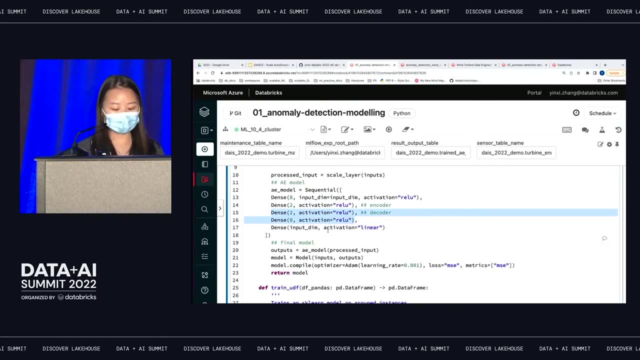 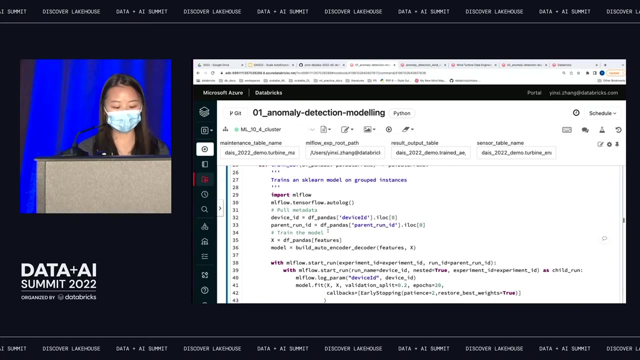 First build an autoencoder architecture. Here I'm just using a simple dense architecture. It has like two layers, So the encoder has two layers, Then our decoder have two layers. The last layer is to reconstruct the input from the autoencoder. Once we have the model being compiled, we get to this training UDF. 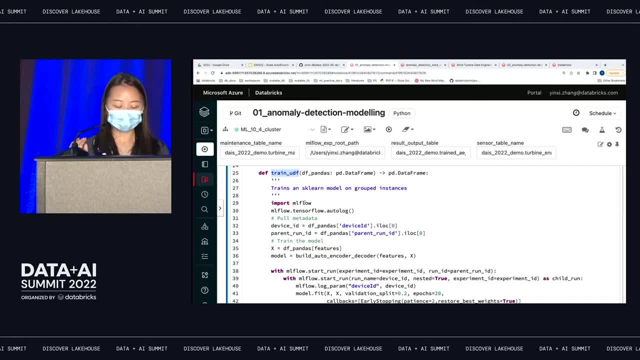 So this training UDF is assuming to work per instance level. So what we will need to provide, we'll need to retrieve some metadata information from the data frame. So we'll need to get the device ID, so which device we are, which device this data set. 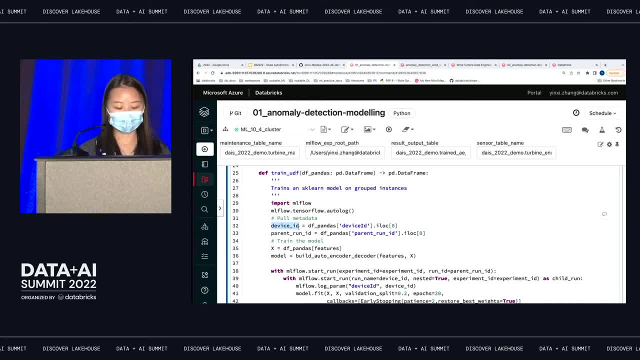 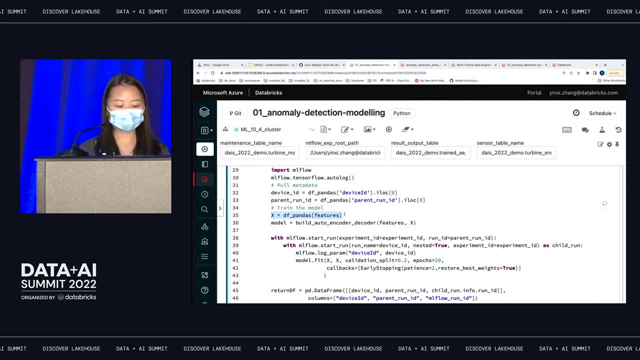 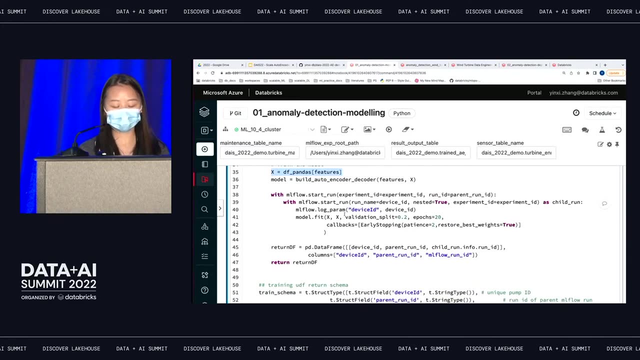 is and we're going to like train the model for this device. So, getting the features and prepare to train the data, prepare to train the model for each training process we're going to. We utilize nested MLflow runs, So all the model training will be scoped in a parent run and each individual device will 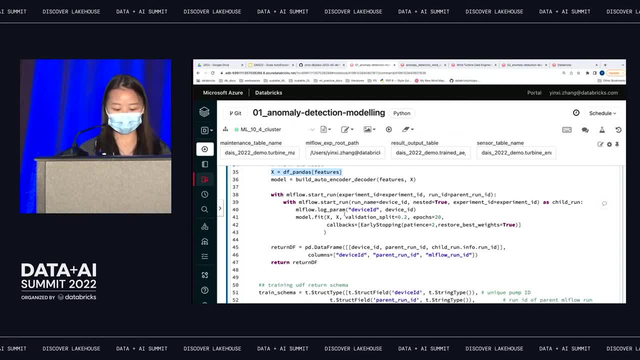 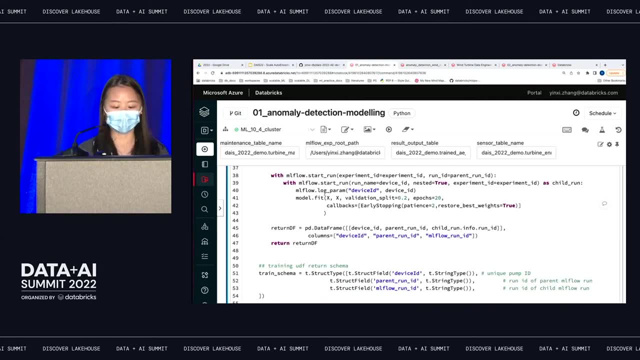 have a child run being Will have a child run representing that device. So when we train each device we'll just log the device information and then train the model and return the device model information. So when we return Here I'm only returning device ID, parent run ID, parent MLflow run ID and the child. 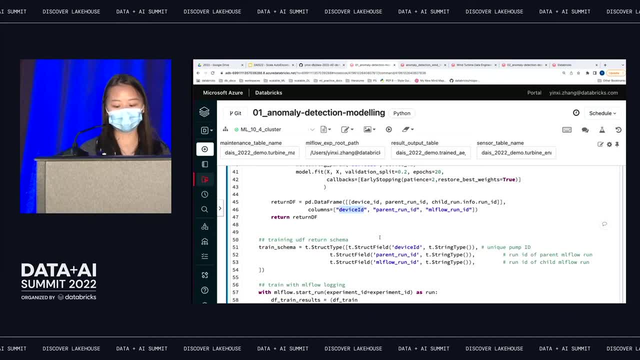 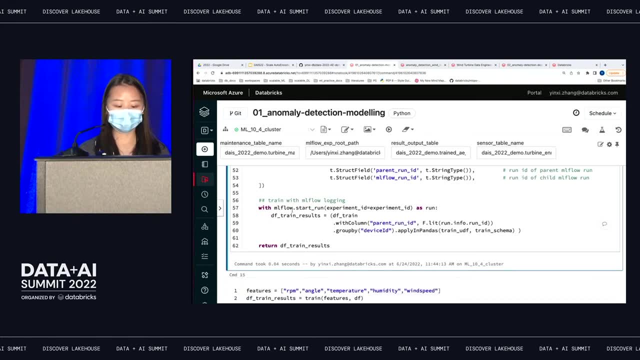 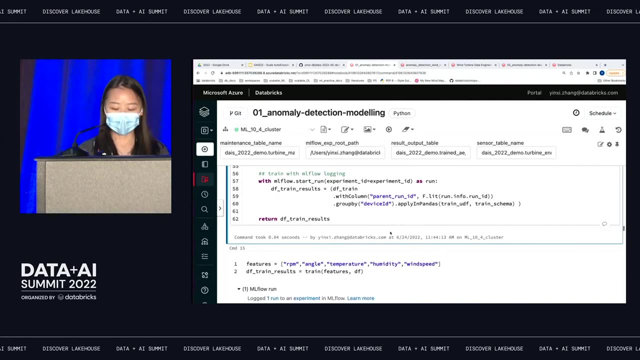 MLflow run ID. Later we'll retrieve the model artifact from the MLflow runs. So here is the return schema and then we can apply the parent run to the overall entire data frame and group by device ID and apply this training function. So you can see here: 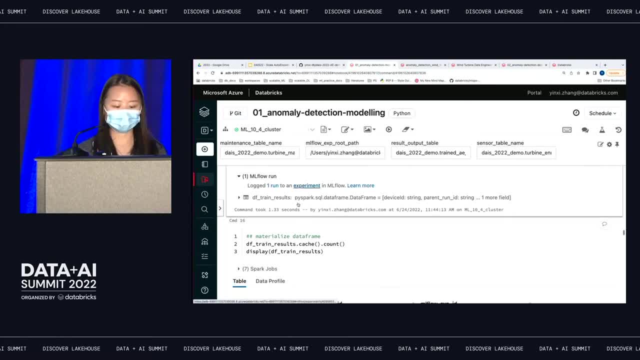 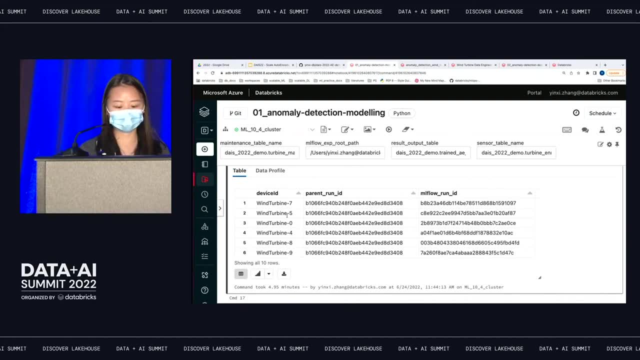 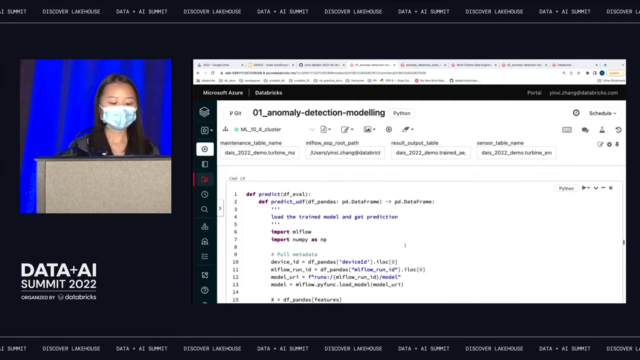 Once we provide Okay, So we have our features and we can get our training results. So training results will be the number of rows you have for this. training result will just be the number of instance you have for your group column And you can see here. we've listed the MLflow run ID per model. 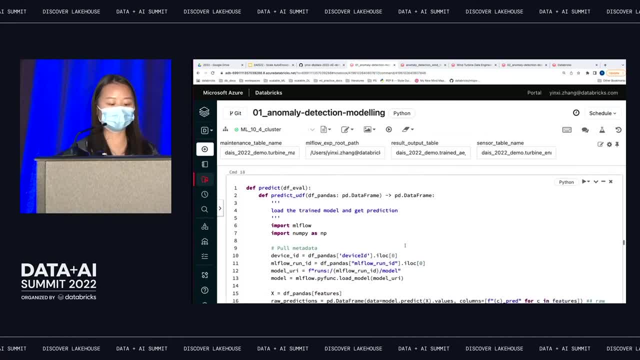 Now we have the information, the model information, we need to use it to generate the predictions, So we can apply the prediction to evaluation data set and also compute the reconstructed error. So we need to have a distributed predict function as well. Same story. 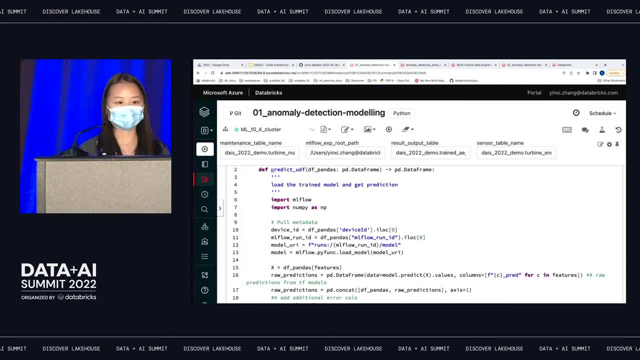 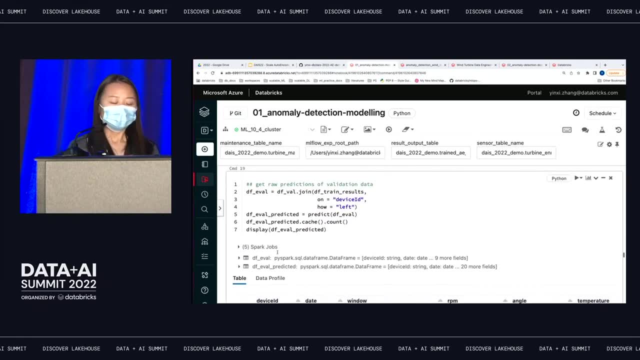 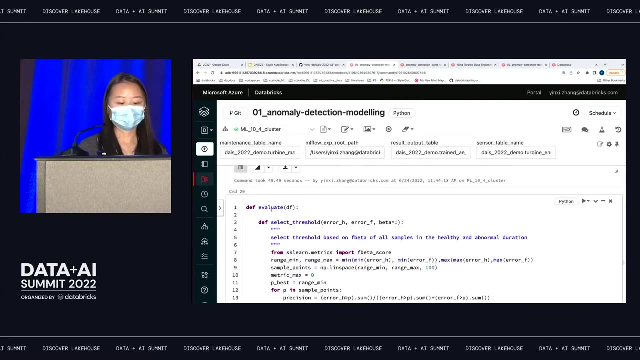 We'll build this predict UDF- that's going to be work on the data frame, per instance- and then do a group by to generate the prediction results. So apply this prediction function to evaluation data And then we can have the prediction. Okay, Okay. 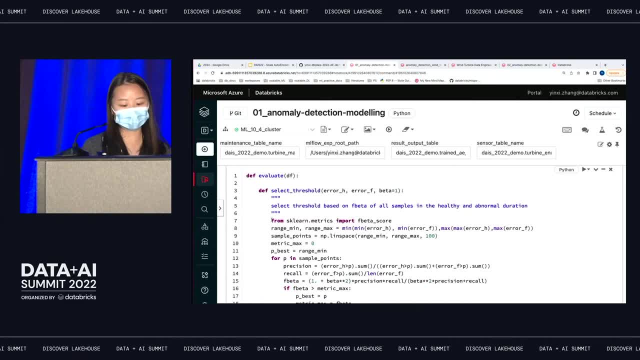 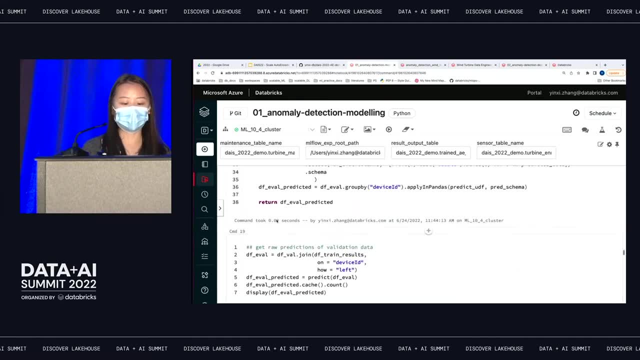 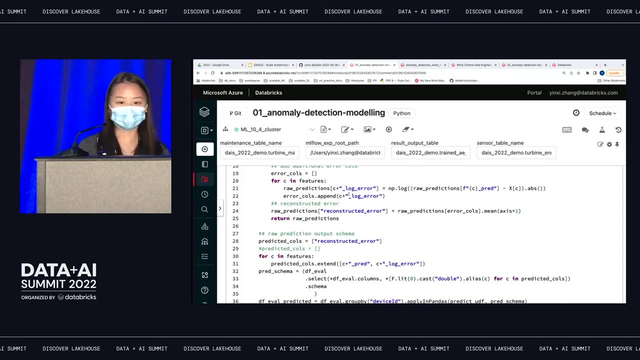 So now we have the evaluation function to choose the reconstructed error threshold. So basically in the prediction function you can see we have the logic how to compute the reconstructed errors. Here I'm using log error per input feature and also taking the total average of all the. 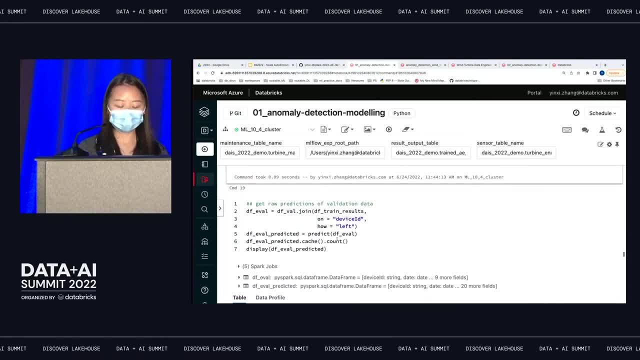 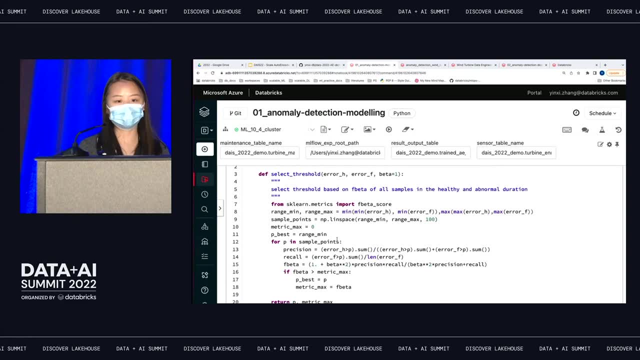 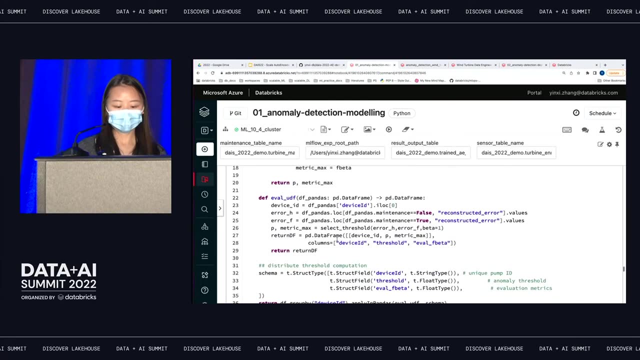 features as the final reconstructed error. Once you have, Once you have the reconstructed error logic, you can choose your threshold logic. Here I'm using a simple F beta score as the threshold for choosing the proper threshold. Same thing This evaluation is going to be applied, per instance, and we use, like Pandas, UDF to do. 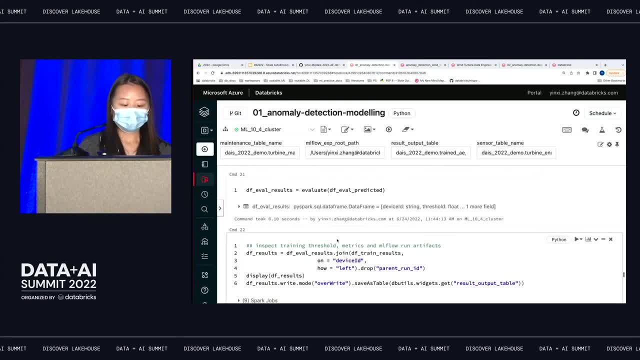 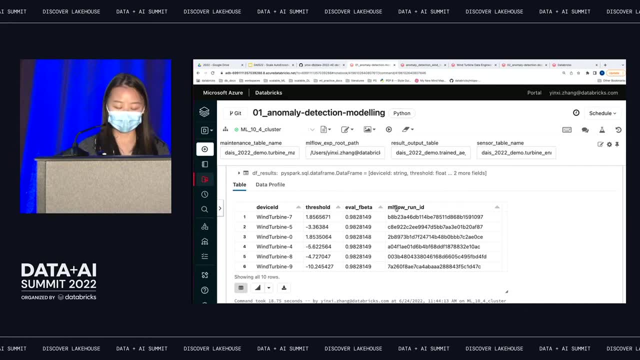 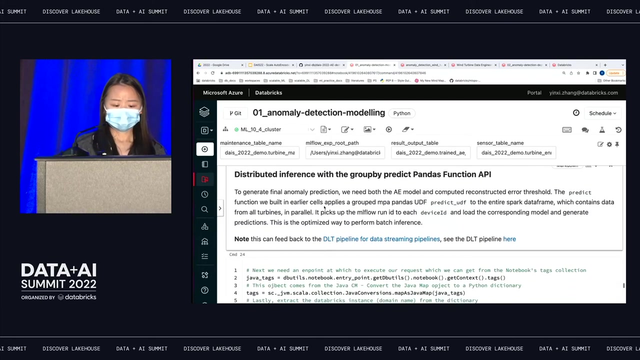 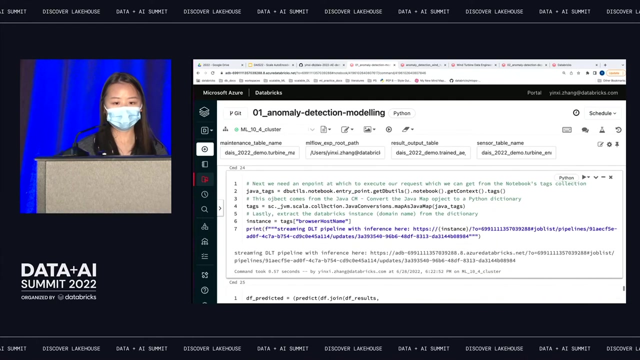 the distributed computation. So in the end the evaluation result will return divisible. Okay, So we have the device ID, your model run ID, but together with your children reconstructed threshold and your final evaluation metrics based on this children threshold. All right, So when we have like a batch inference, it's quite straightforward to use the predict function. 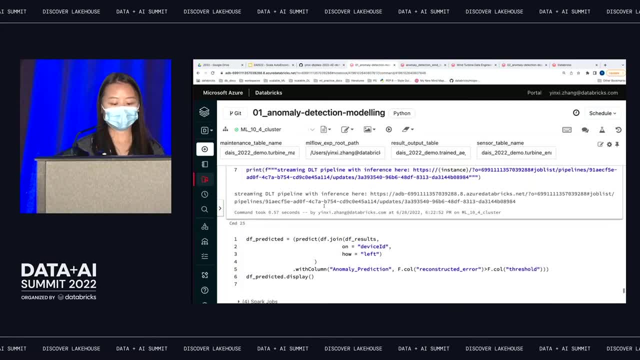 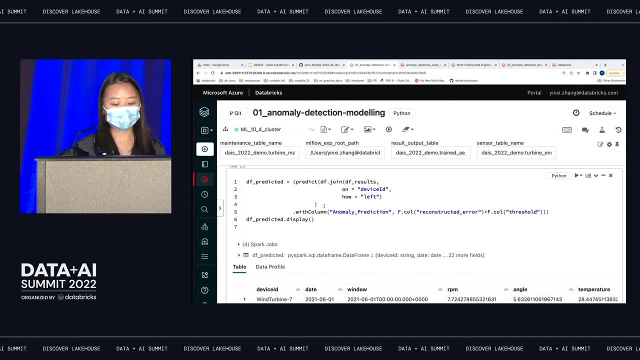 we just defined. Okay, So now we'll go ahead and we'll record the data on the device. So the first step is to record the data based on the device ID. We'll do that on this model. This model is a much smaller model than 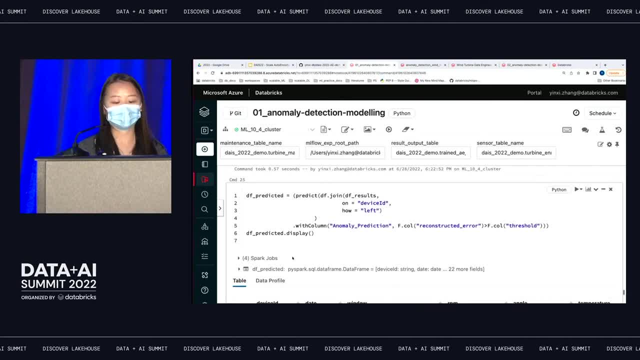 This model is a much smaller model than the device I mentioned earlier in this notebook in inference pipeline, and this way we'll be able to generate prediction. We'll be able to generate final predictions based on the entire batch data, So this batch data have information from all the turbines and then it will find the proper. 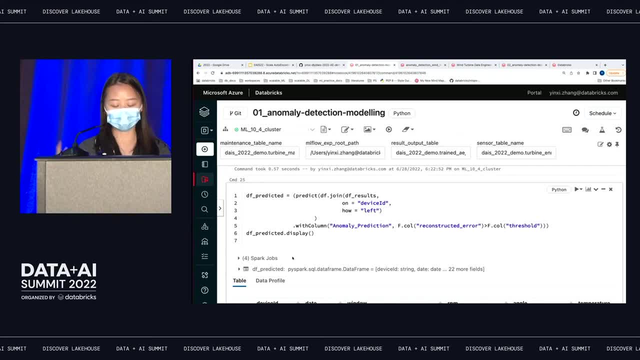 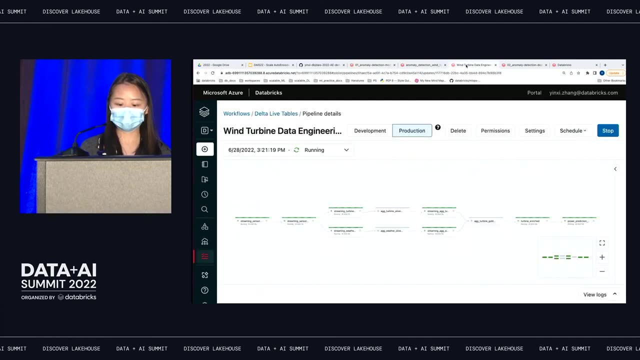 model based on the device ID column and then select the right model based on the MFL index of the device flow run ID and apply the model prediction from there and create the final anomaly detection label. And in the streaming case we can take a look at the DLT pipeline. 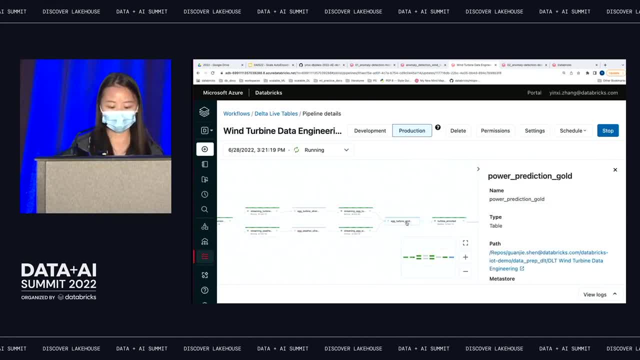 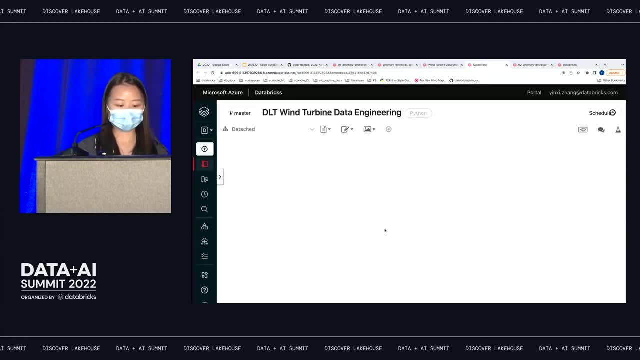 So the last step here is to generate a power prediction, and we can see from the DLT pipeline notebook that we apply the same predict method, using the group by UDF to attach to the streaming pipeline and generate the predictions for the stream batches as well. 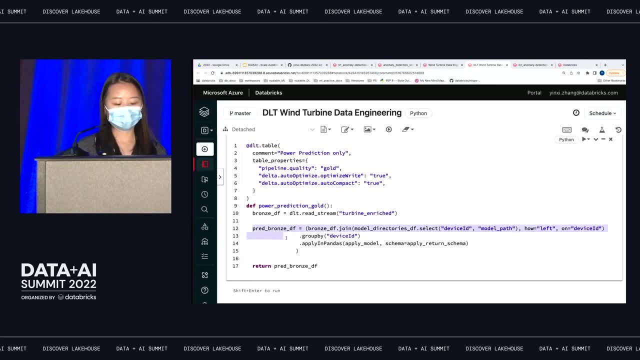 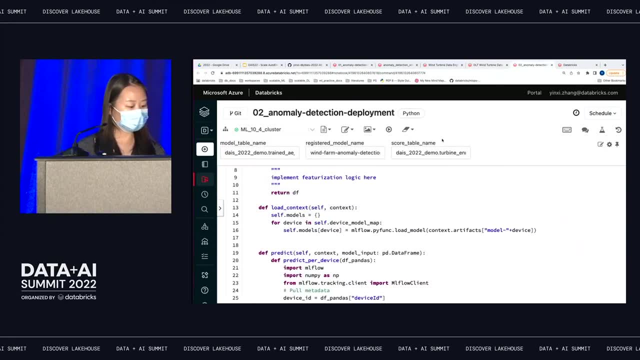 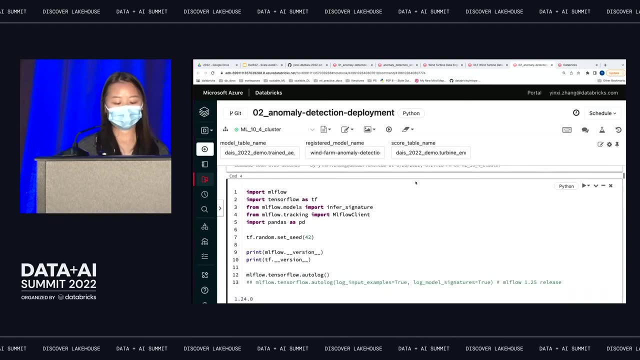 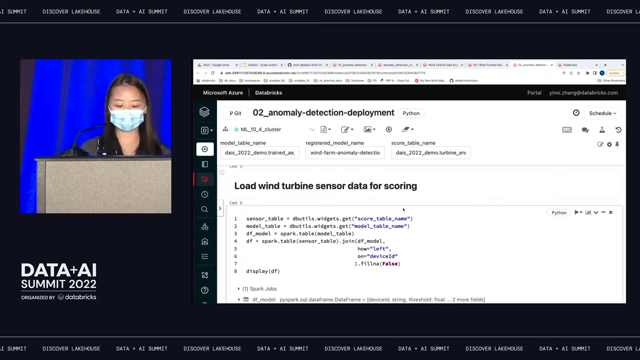 So this is the prediction step added to the entire streaming pipeline for streaming inferences And in the case of real-time deployment, what we are doing here is we're going to build a customized MLflow pyfunc model that will ensemble all the models together. 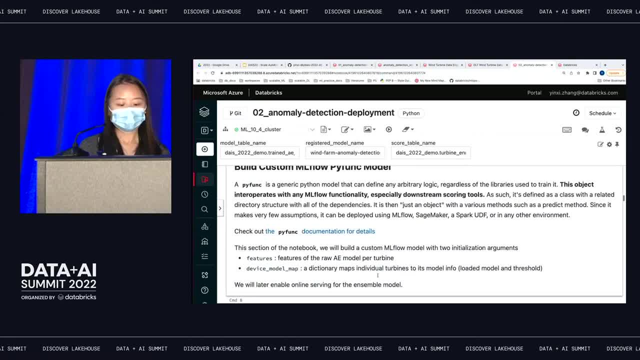 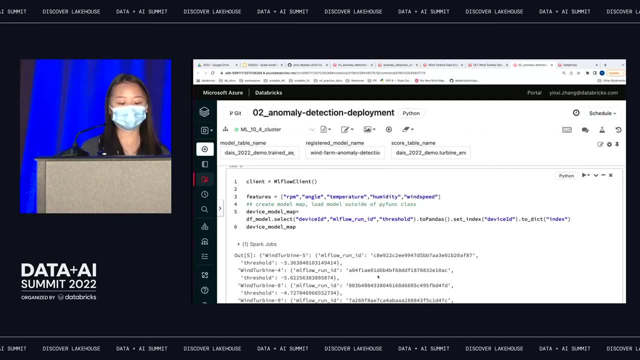 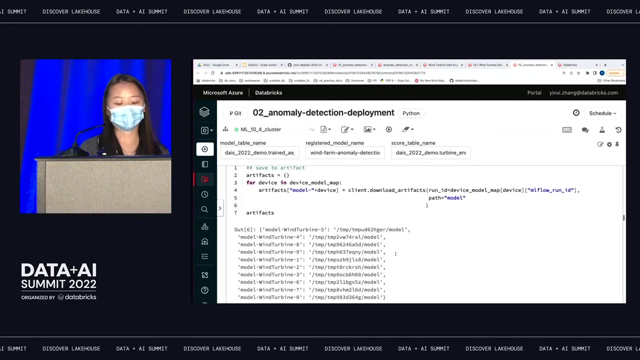 and create a REST endpoint out of that. So let's get to the model preparation. So we'll first need to build some model artifact. We create a map which will map the device ID to the model artifact and use the model artifact as context for the MLflow pyfunc. 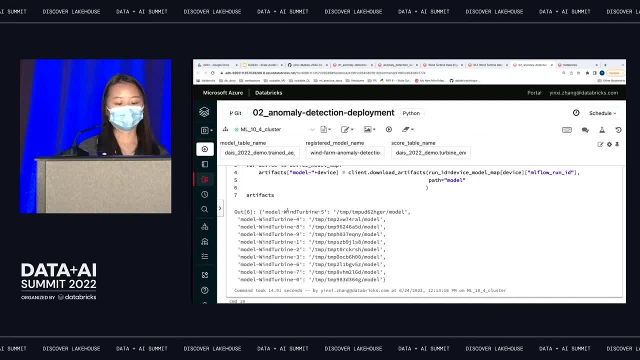 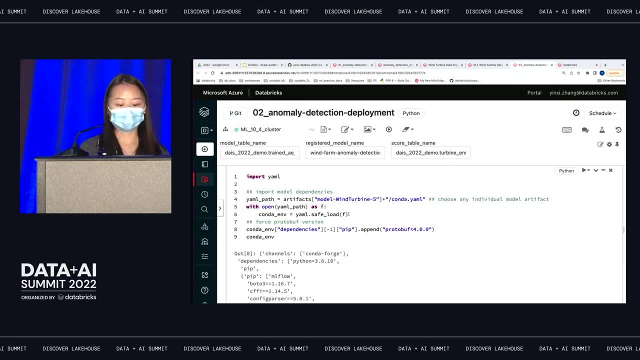 So you can see the artifact represents your model per device and the model artifact location, And we also need to prepare the dependencies for the dependencies for the ensemble customized model. Here there's only a slight change with respect to how the model is arranged and logged. 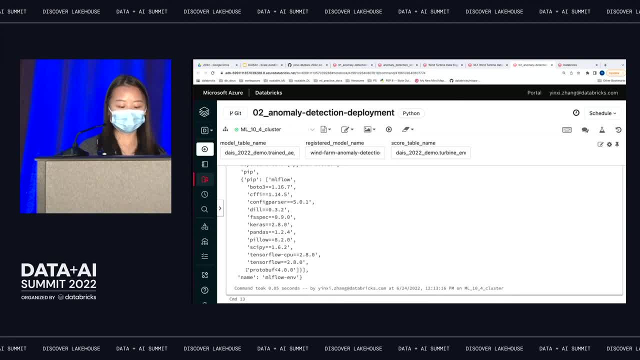 It's this protobuf version has to be earlier than 4.0 to avoid like a serving issue. And then we start to build this customized MLflow model. So this is going to be an inherited instance from MLflow, So we're going to build this customized MLflow pyfunc. 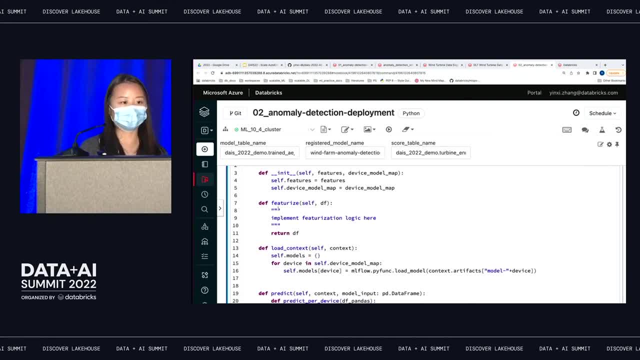 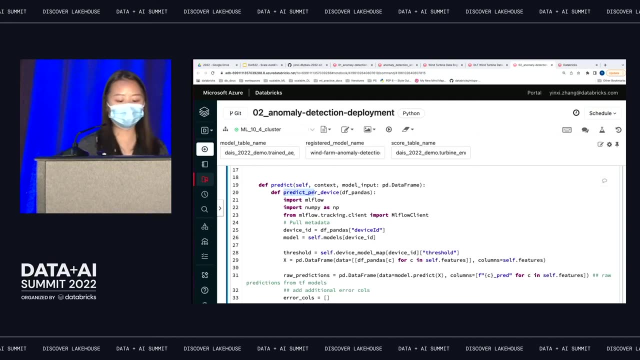 Python model, You can implement your online featurization step within the model as well, And then the load context is basically loading the model artifacts we have prepared ahead of time, And then in the prediction function we can predict per device and then use: apply. 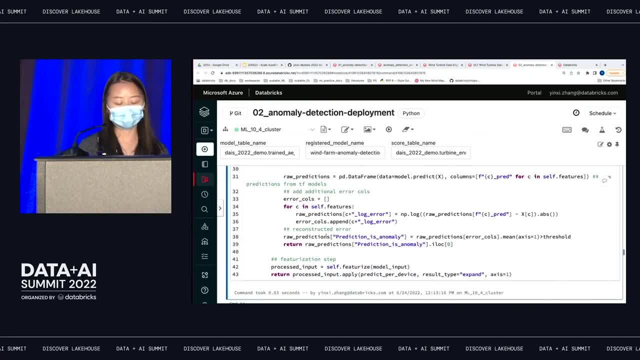 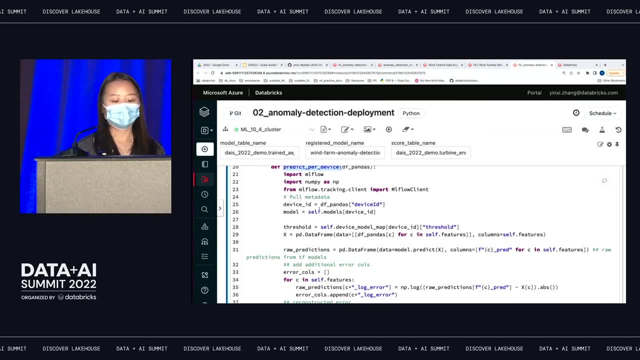 pandas apply function to generate the final prediction result based on each device ID. So same, So similar logic here within the predict per device we need to understand, retrieve the device ID information and then use the artifact we provided to select the correct model. 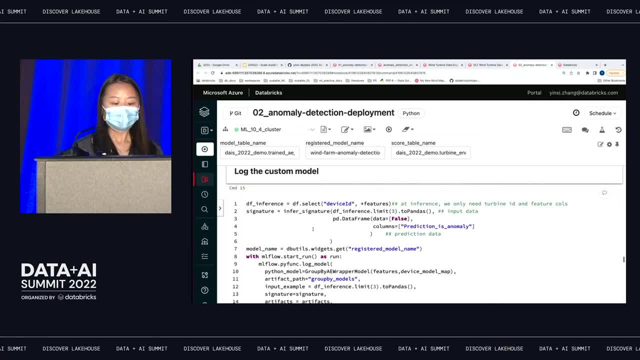 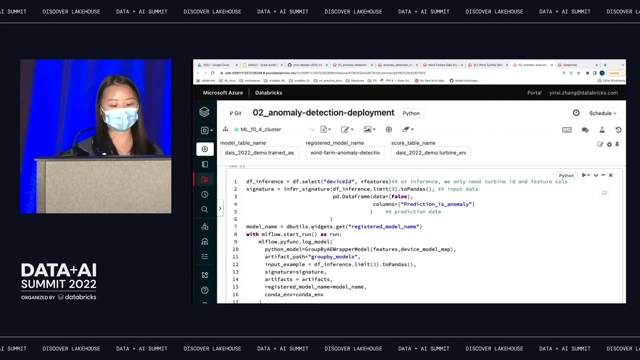 and then generate predictions from there. All right, So once we built this customized model class, we need to create an instance out of that class and log this customized model. So we're going to use, we're going to use, we're going to use. 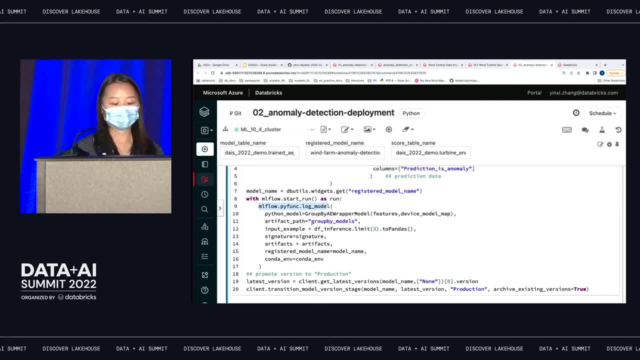 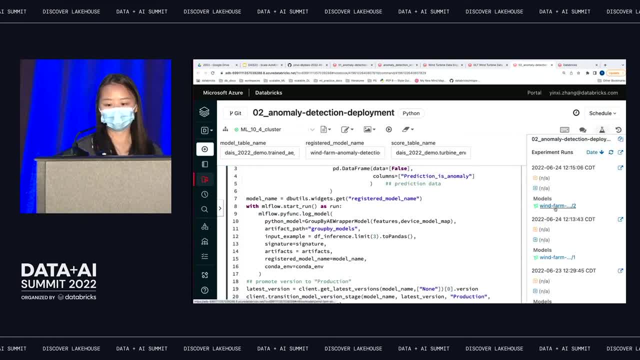 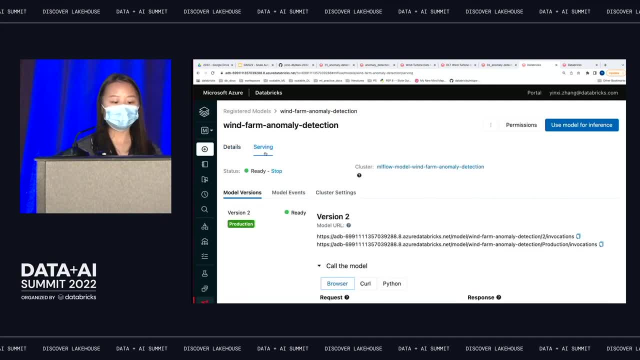 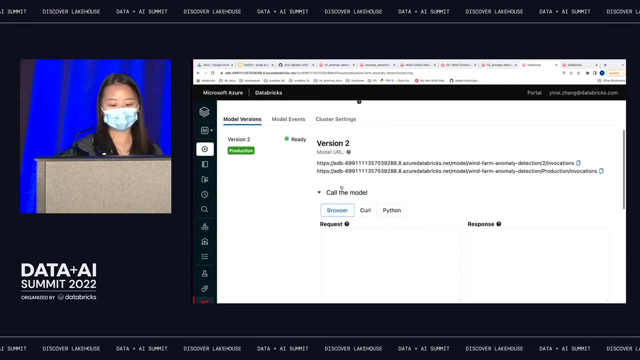 In the end you can see what has been logged here is in the model registry And if I get to the model registry page we can build like a serving endpoint from this model. I have already like enabled the serving where we can see it's the endpoint is ready. 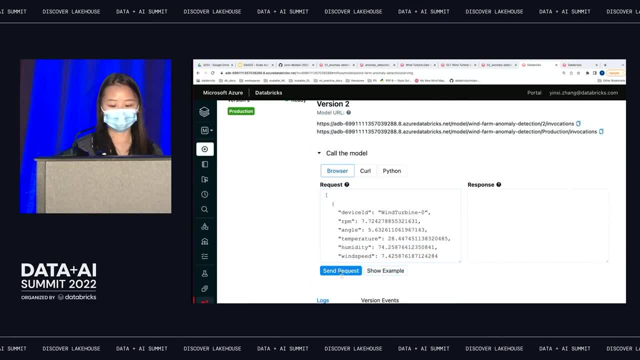 And we can send a sample request to get a response out of it. And you can see here, it does take the device ID information as input. So if you have a mini batch of data coming from all the devices, it will be able to generate the predictions for each device. 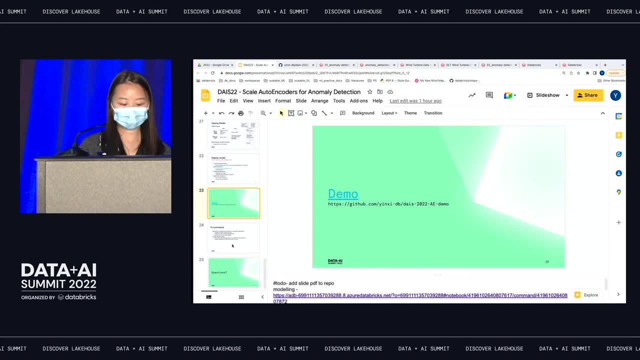 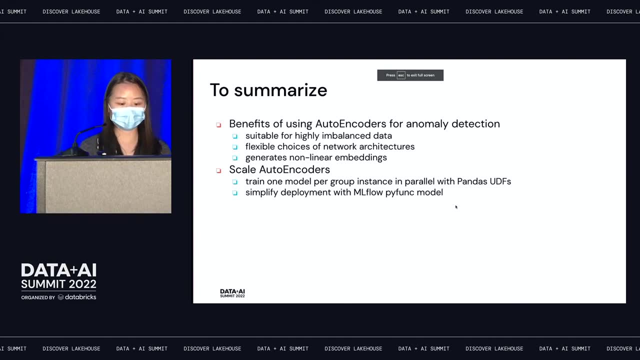 All right. So that's all about everything about the demo. And to summarize, the benefits of using auto encoders for anomaly detection is that it is suitable for highly imbalanced data. You have flexible choices of network architectures. It also generates nonlinear embeddings. 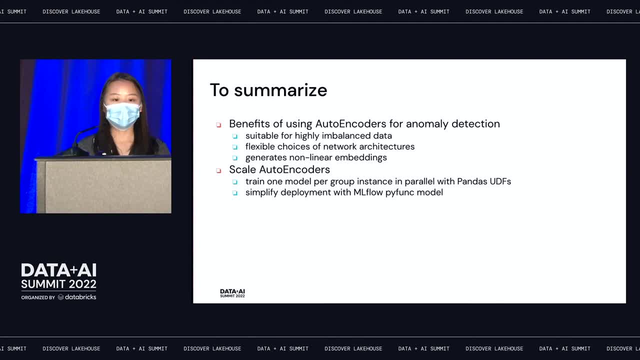 which can be used for downstream tasks And the way to scale auto encoder solutions. for training, we can train one model per group instance in parallel with pandas, UDF, And for deployment, we can build MLflow Python models to assemble all the models into one. 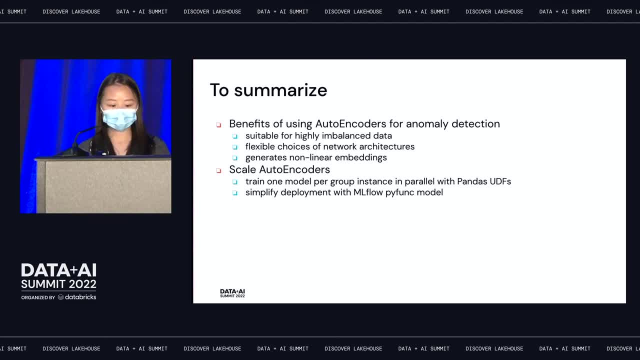 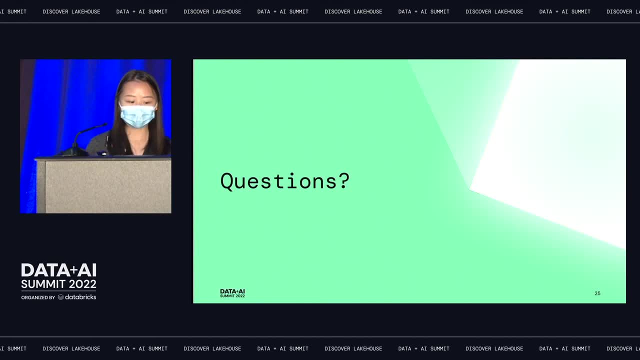 and deploy that single model as REST endpoint, And it can also be used in batch and streaming pipelines as well. All right, Any questions? I think I'm running out of time. Shee, That was a great presentation. I appreciate it. 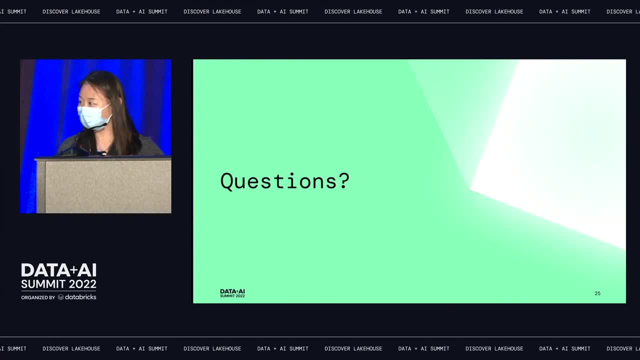 So many questions out of the podium. Yeah, We'll spend a few minutes on questions. Hey, So you said when you're training a model per group, right? Can you please clarify how you're going to feed in the abnormal and normal data at every group? 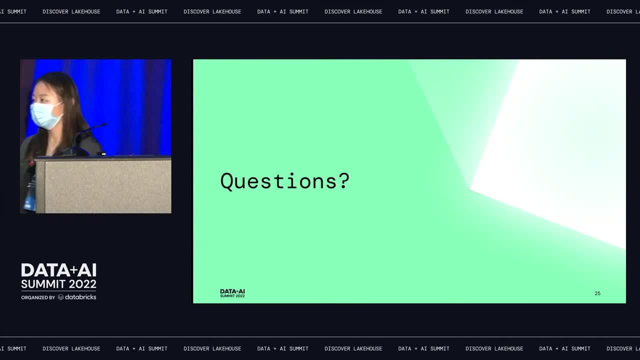 You're going to do that, Or can you please clarify that? How is that going to work, right? Right, So the training is basically the model. fitting is basically on normal data only, so at each step the process is distributed, so the chain udf will do the modelfit. 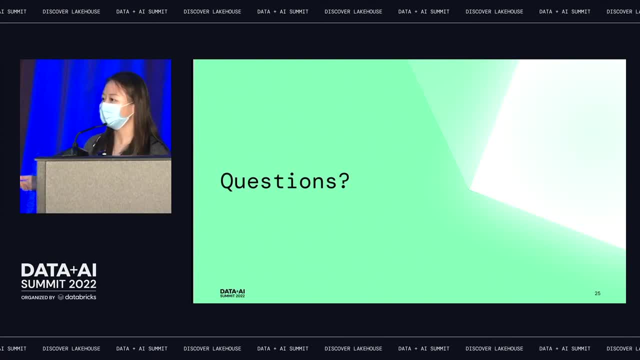 and that's going to be distributed for the entire group at the same time. once you have the chain, the, the model being chained, we're going to use predict and evaluate with the combination of normal and abnormal data to select the threshold. so the evaluate and predict function will also be distributed using the pandas udf. 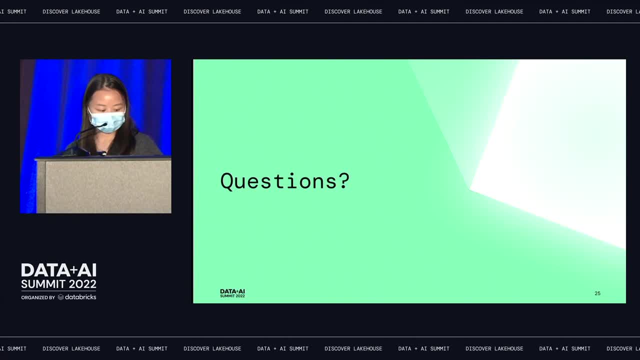 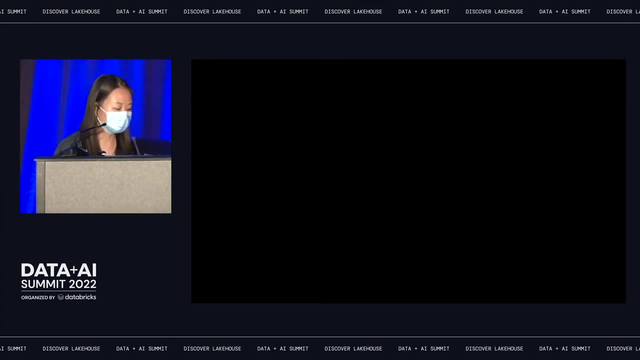 thank you, okay. one last question, hi, a quick one. so when you apply in compendus and you choose group by field- so it was device id- what if you have imbalance data? so for some device you have, like i don't know, gigabytes of data, terabytes, and for some you 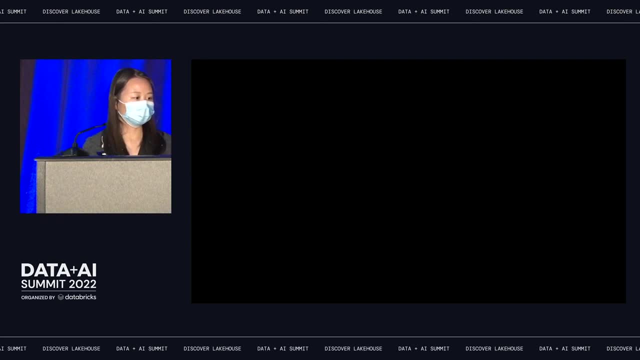 have, like i don't know, 10 nodes and like: how do you, how is it possible to balance that right? that's a great point. i think it will have some impact on the performance of your parallel training. in that case, maybe try to pre-process what this is like, thinking out of my